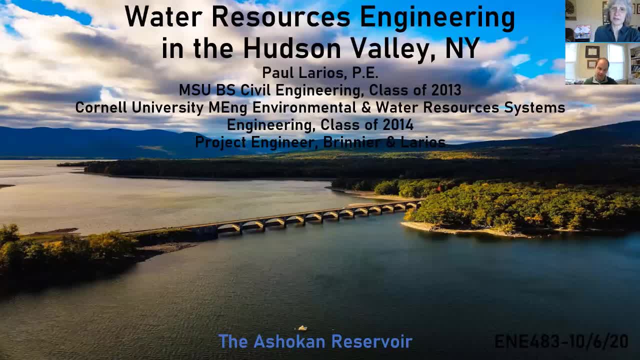 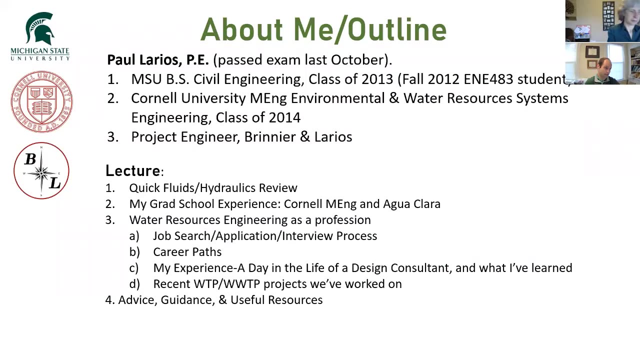 It's their largest water supply and I'm going to tie that back in on a few of the projects I'm working on or I've worked on. let's see a little bit about me. Yeah, class of 2013.. So 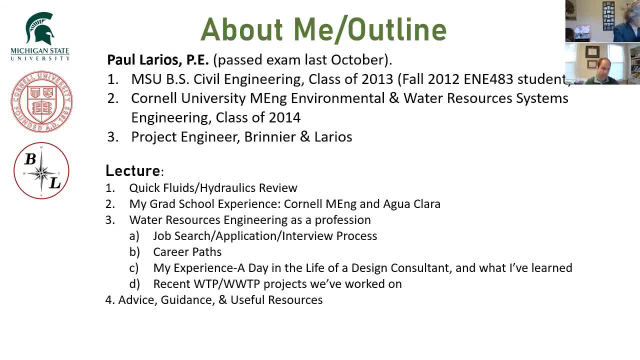 seven years ago I was sitting in your seat taking 483.. And then I did a one-year Master's of Engineering program at Cornell, which was just 30 credits, Of course work two semesters And then I went to work. So it's been six years of working as a design. 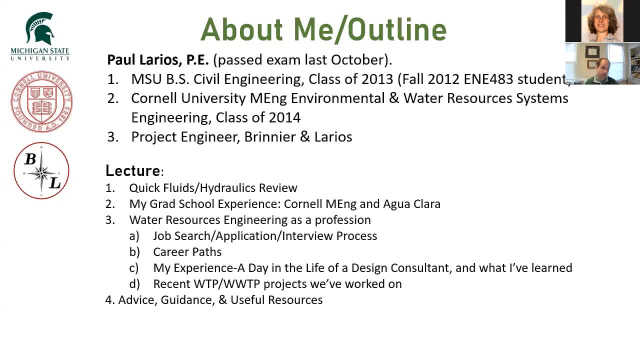 consultant at a small firm that I'll get into more on. So I promise not to get too technical, but I want to review some basic fluids to start, because anything you learn in this class kind of needs to be paired with fluids and hydraulics to effectively design. 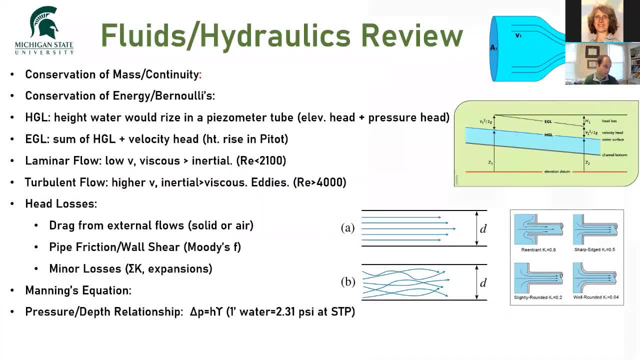 water and wastewater processes. So first, conservation of mass and continuity. Does anyone know the equation for this? Anybody? There's a graphic. This is the MDOT stuff we just went over, right, Dr Marsden. So conservation of mass just is, you know, flow in equals, flow out, Area, times, velocity. 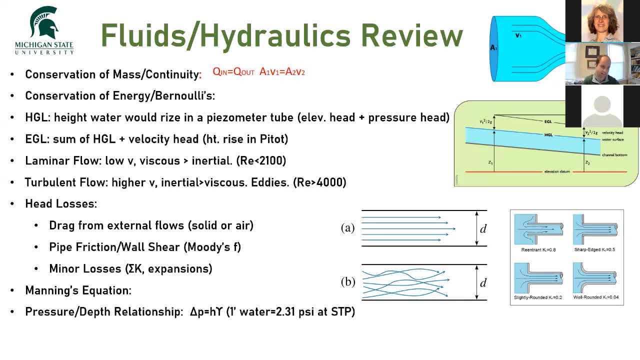 stays constant. as you can see in the graphic to the top right, V2 is going to be larger than V1 because it's a smaller diameter and a smaller cross-sectional area. So that's a very important concept, Followed by Bernoulli's equation, which is: 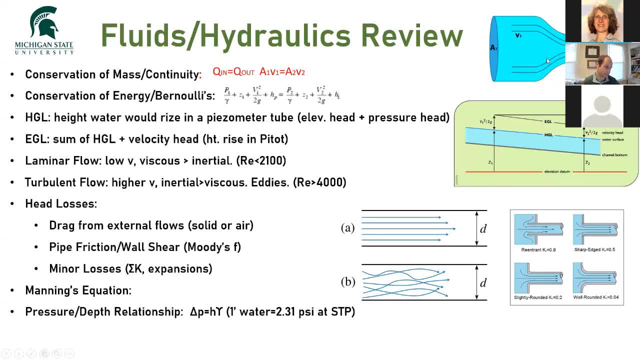 conservation of energy. And you see terms here for head added by a pump and head loss is weather friction minor. So next, hydraulic grade line, That's the height the water would rise in a tube, Elevation and pressure head. So this is important for plants mainly because 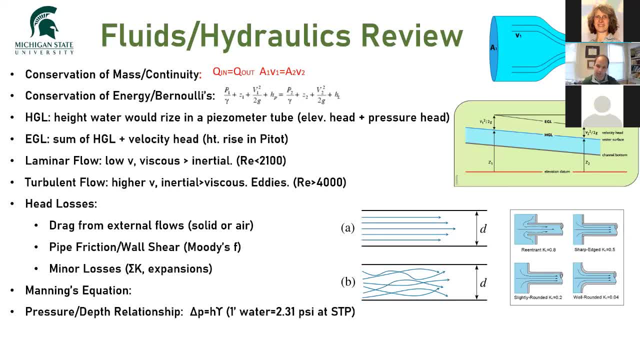 any time you do a plant or even a sewer pipeline, we track the hydraulic grade line through the entire system and do a hydraulic profile. So it's very important to know where your water surface level is, And that's as you can see on the graphic: to the right water surface is hydraulic grade line And then 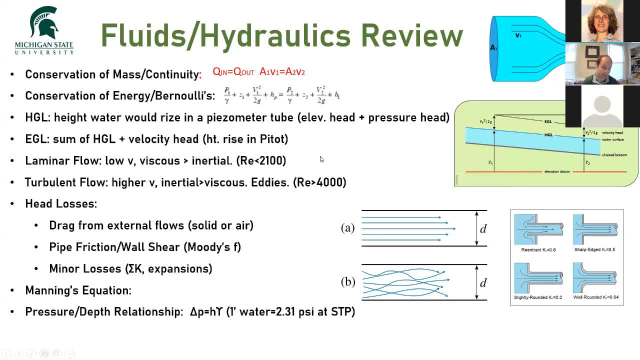 the energy grade line is just adding the velocity head to that. And then a couple of flow regimes: laminar versus turbulent. In laminar flow, at lower velocities we had have viscous forces dominating rather than inertial forces, lower Reynolds numbers. 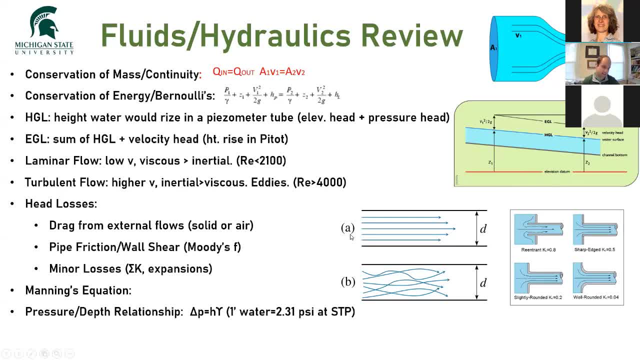 So laminar flow would be case A here, with the undisturbed streamlines, and turbulent flow is obviously where they are deviating and that's an extreme case, But then we have head losses. So we can see a lot of discrepancy and this is the main reason why it's important to track. 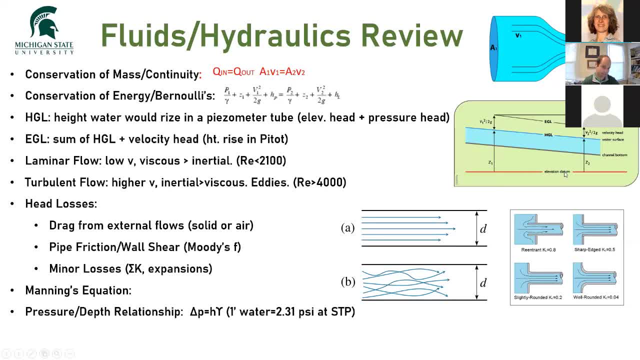 through the water. So then we have drag losses, which are also very important to track through a plant, And it affects your hydraulic grade line. Drag- that's kind of rare, but we're always what you call major losses: pipe friction and wall shear. Use Moody's diagram, I'm sure. 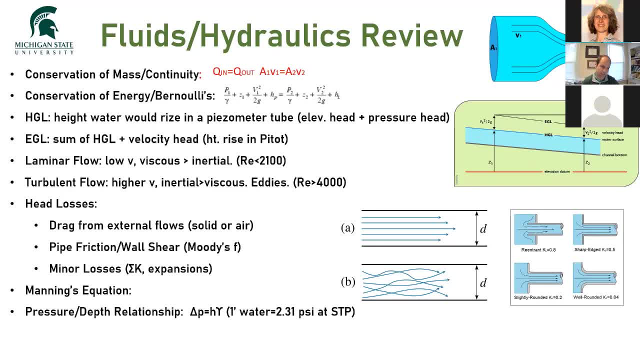 you guys learned in fluids And then minor losses you can see are caused by, you know, sudden contractions, entrances, like in this bottom right graphic where the streamlines are disturbed. that is, showing your energy loss through it, through an entrance and the corresponding K values. 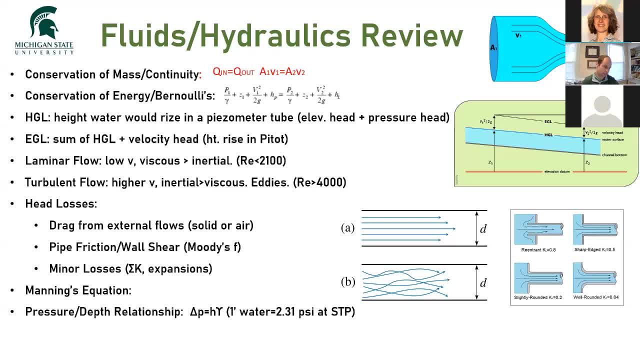 which are summed up to get your total minor losses, which hopefully you can keep your minor losses minor Manning's equation- I'm sure you all know that that's mainly used for open channel flow, pipe flow and then pressure versus depth. So with constant density pressure is going to increase as 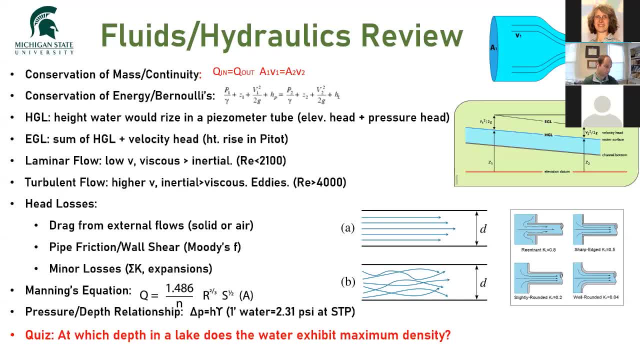 depth increases underwater Quiz. At which depth in a lake do you guys think the water exhibits maximum density? Yes, Everyone's on mute here. No guesses. you can use chat with a question mark, Anyone else? Yeah, I thought the density was constant. 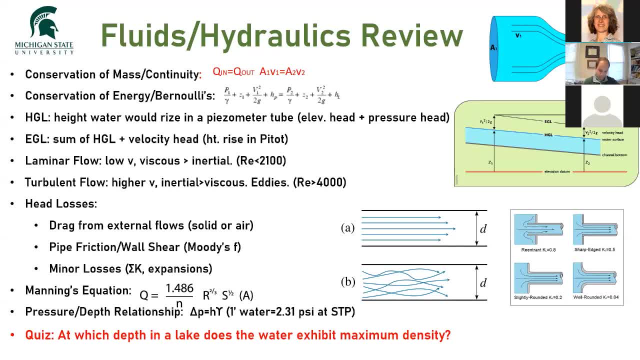 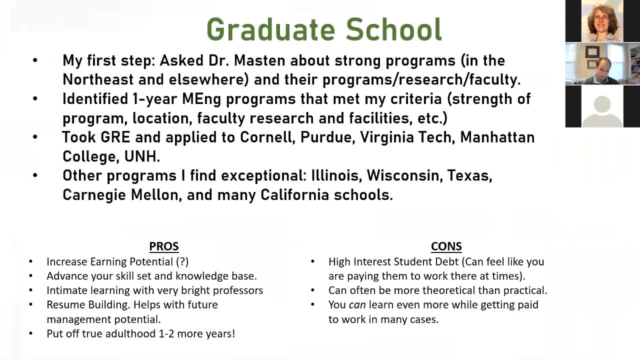 throughout, like all depths of the lake, No, so density is gonna be greatest at the bottom of the lake, where pressure is the highest. So, graduate school: I was pretty much dead set on grad school throughout undergrad So I knew I was interested in water. 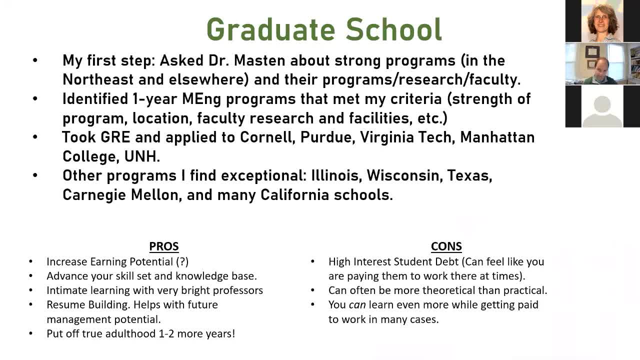 and wastewater treatment. So my first step was asking Dr Mastin. because I knew she was familiar with other programs and faculty and research and their programs. I knew I wanted a one year master's in engineering program So I based on Dr Mastin. 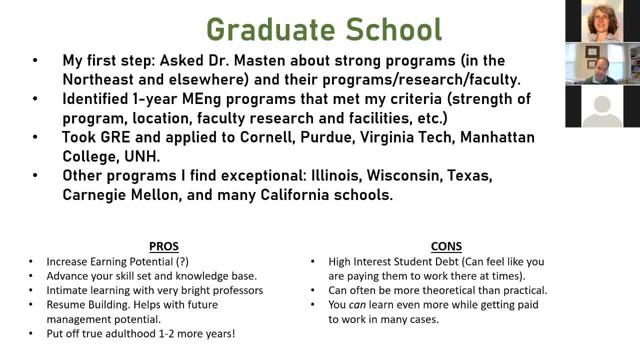 I had a list that I had brought her and she kind of solidified it for me And I applied to Cornell, Purdue, Virginia Tech, Manhattan College and University of New Hampshire. I think I got into all of them. I took the GRE. 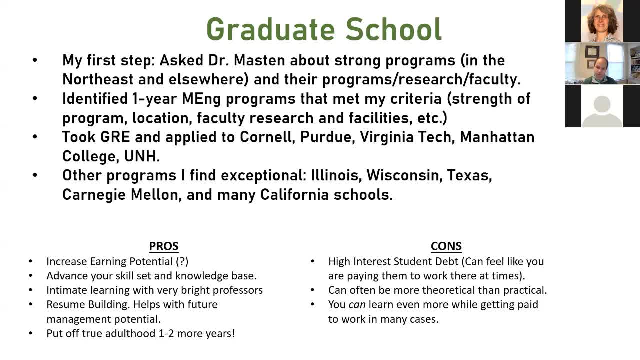 I think that's being waived by many schools this year. If any of you are, I'm looking to apply And similarly, if you're not- I mean if this isn't your what you wanna specialize in- you could. if you wanna do geotechnical. 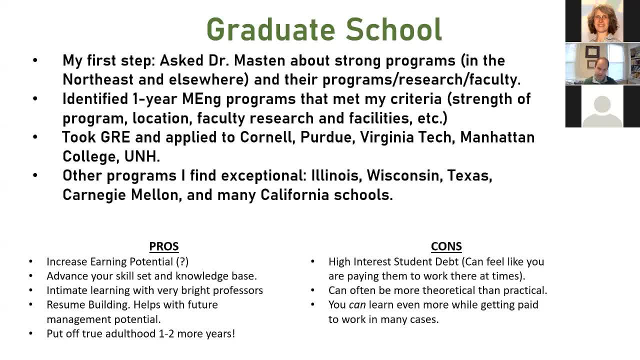 you could. I mean, I'm not sure who the department, maybe chatty or- but your professors can definitely help you find strong programs and MSU has strong programs. I know they have a, a five-year master's, but you probably would already have to be enrolled in that. 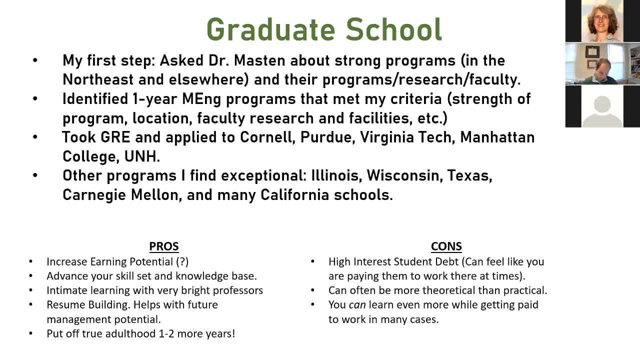 So pros and cons of grad school that I found it can increase your earning potential, though I found that right off the bat it did not. I interviewed at two firms, one in New York city and one in Westchester, right outside of New York city. 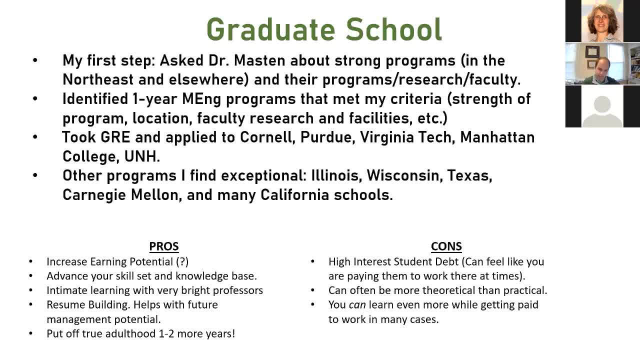 where the cost of living is very high And I was kind of a, you know kind of a- I just graduated with a master's from Cornell and I was expecting to get compensated for that And I was still getting offers around the same area. 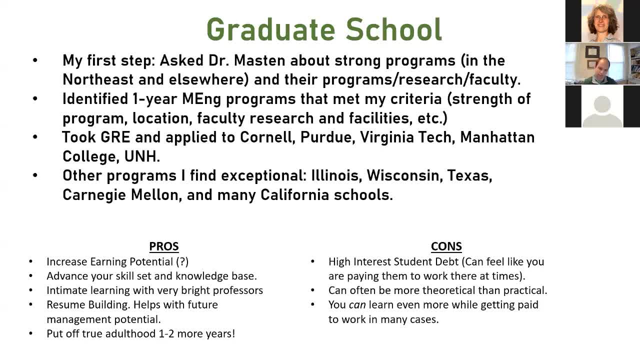 that I could have gotten with my bachelor's, Though I do think it increases your earning potential and your potential for management roles down the road, And you learn a lot of valuable tools. Advance your skillset and knowledge base. learn the newest skills. 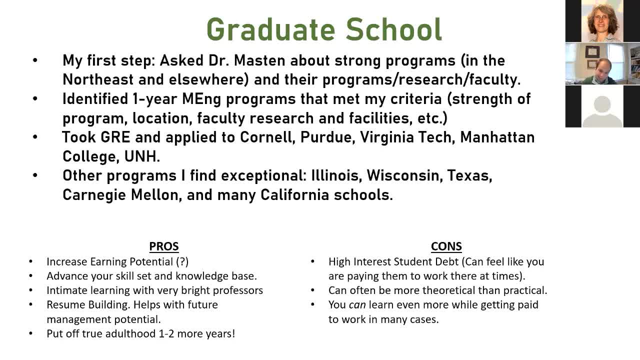 intimate learning with very bright professors. That was the highlight for me. I mean, some of my professors were just, you know, so great to learn from and you learn new ways of thinking and solving problems And it's good resume building. 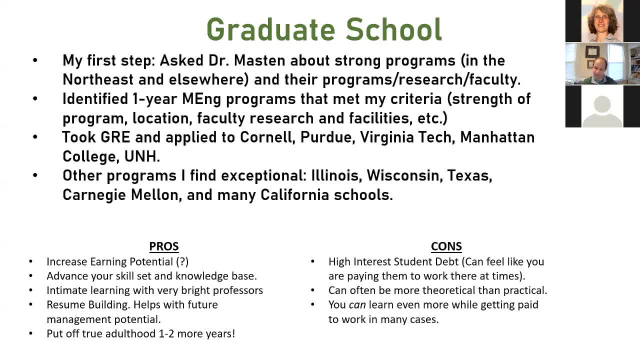 And you can put off true adulthood for another year or two. Half joking there, but some cons. Student debt is very high interest 7% plus in most cases, and that can cripple a lot of people, especially non-engineers, where you're not. 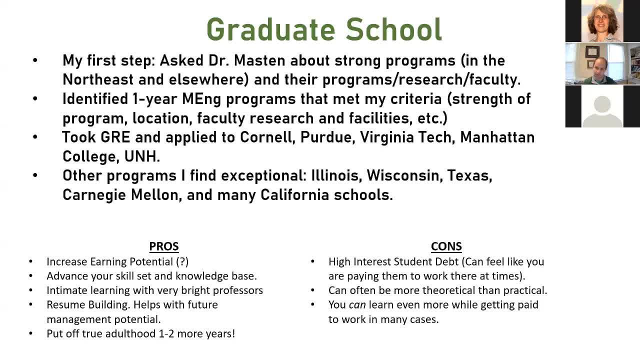 kind of come out with the job guaranteed and a good job guaranteed, but I would say that all of you can have a good time. I mean, I had to pay my teachers at the school, business school's International student loan And that's pretty much my whole life. 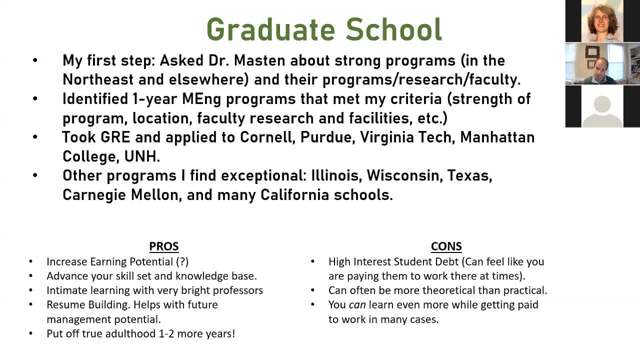 And I don't think I'm gonna go into all of the details that I have to give you on my slide. I'm pretty sure I have some of those information as well, But I think, at the end of the day, that that I was paying like 600 a month. 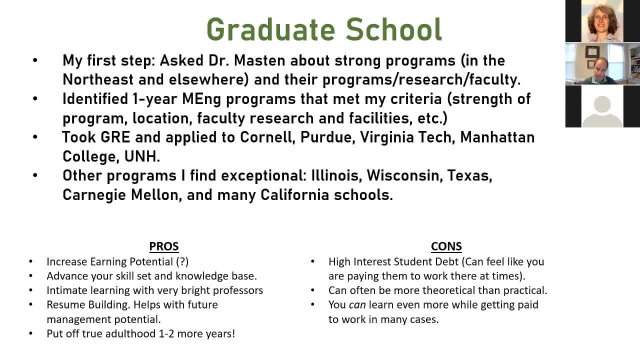 I paid my not pretty quickly. Last year I paid over a thousand a month just because it's such high interest. you know professional development programs are aiming to get rid of that. still, I could tell you Cornell: I spent hours and hours coding and MATLAB and I 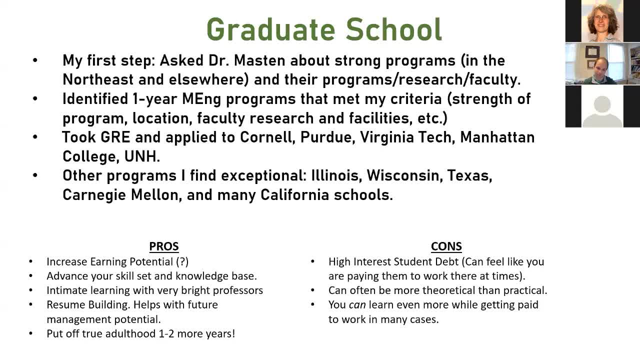 have not used MATLAB since, so some of it is still very theoretical, but I did learn a lot and I think that you can learn even more in the office while getting paid to work in many cases and more practical knowledge. I don't regret going. I just that's my biased perspective of the pros and cons, so take 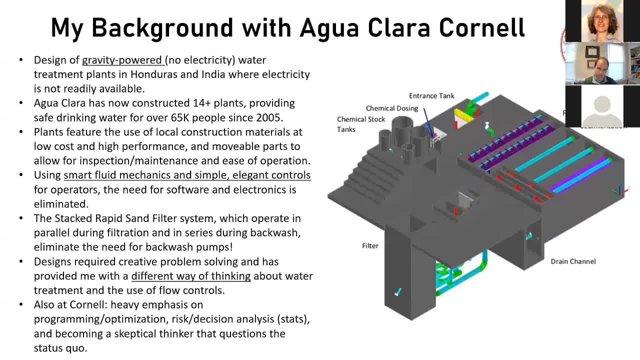 that with a grain of salt. so my main draw to Cornell was the Agua Clara program, which is awesome. I mean they designed gravity-powered hydraulic water treatment plants in Honduras and India in areas where there's no electricity available. so in order to do this it, you know it needs to be completely. 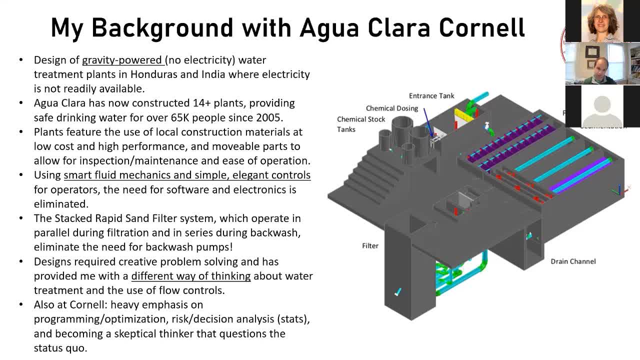 gravity-powered and you need to come up with very creative solutions using smart fluids and simple, elegant controls. they've now are over 14 million units of water in the state of California and they've done a lot of work to get that to the state of California and they're still working on. 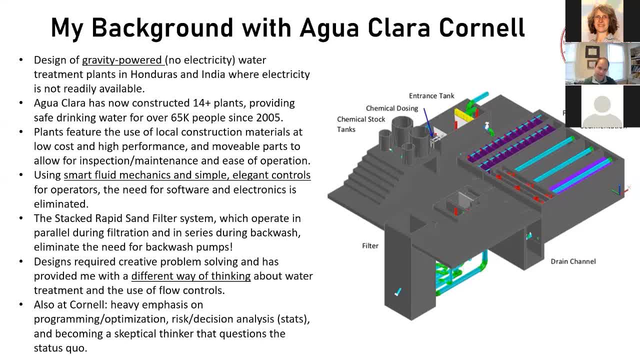 getting that to the state of California. so I think, you know, I think that's an amazing opportunity. we'll have to see if we can get it to the state of California and we'll have to see what happens. but yeah, I think we've got a lot of people. so that's not going to be a problem for us to get that to the state of California and we've got a lot of people that are looking for that and we'll have to see. It's much more simple than a conventional treatment plant. The filters: I don't know if you guys have gotten a filtration yet. 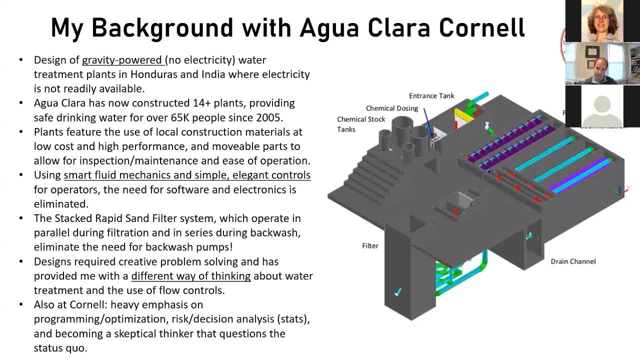 but the filters are quite the technology. I'll get into more in the next slide, but they eliminate the need for backwash pumps using their stacked rapid sand filter system. This program really helped me think differently about water treatment and the use of flow controls. 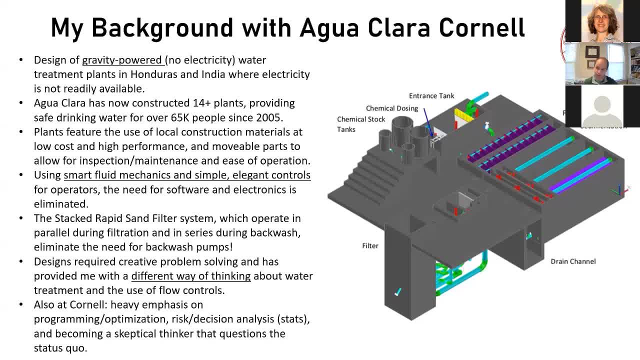 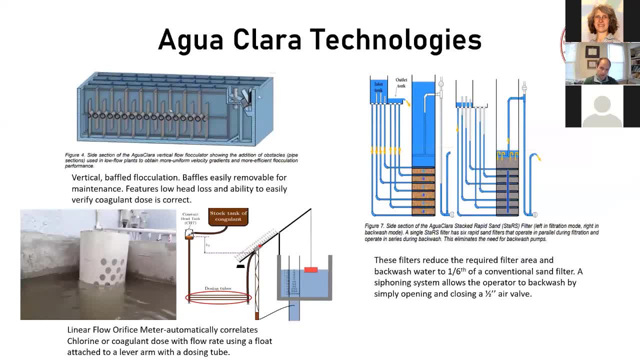 I still use that way of thinking and try to apply it to conventional treatment when possible. Here's some of Agua Clara's treatment processes that are. I look at them as inventions. They use vertical baffle flocculation where water goes up. 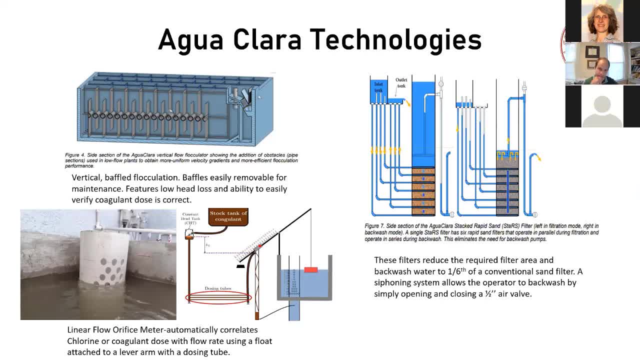 and down through these PVC baffles that are easily removed. This really ensures adequate mixing and it's low head loss and it's all hydraulic. You're mixing without using any type of rapid mix system. The linear flow orifice: they have a few different dosing mechanisms like this: 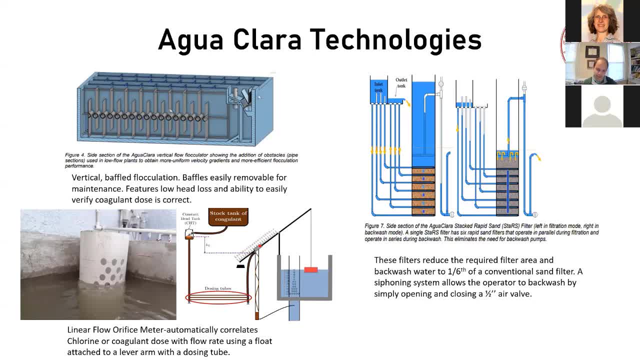 that you can automatically adjust the dose of a coagulant or chlorine based on the flow rate in the plant using a float valve and a lever arm that just changes the dose automatically. Then, on the right, here is their filter filtration system. It reduces the filter area needed by one sixth. 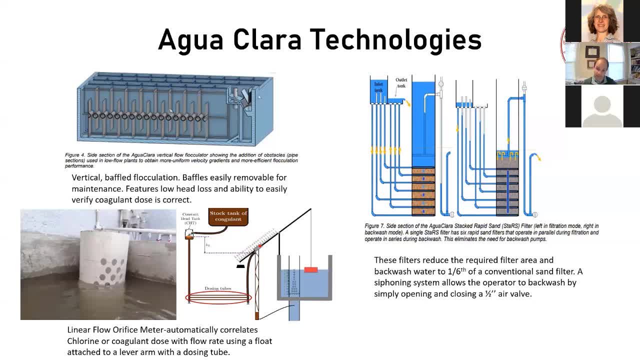 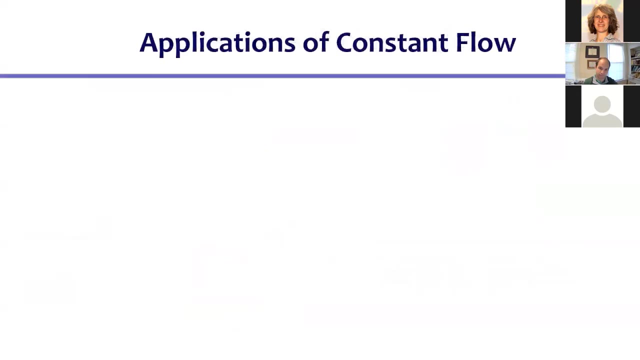 which is huge, And they use a siphoning system that allows the operator just to open and close a half inch air valve to backwash. And that is. those are the three that stuck out to me. So here are a few slides that I've taken from maybe my first or second Agua Clara lecture. 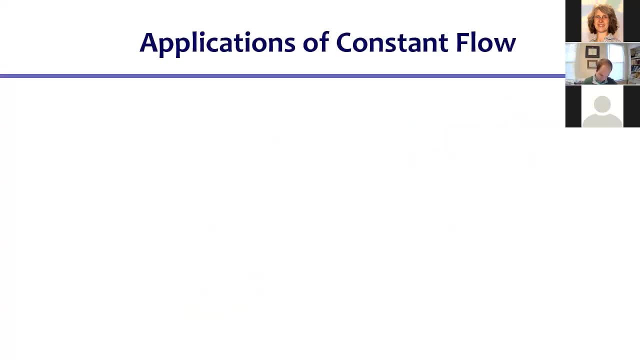 just to kind of get you guys thinking that way, I have a link to the whole PowerPoint at the end of this, at the end of my presentation, which I sent to Dr Mast and I think she can share with you. So so, constant flow. 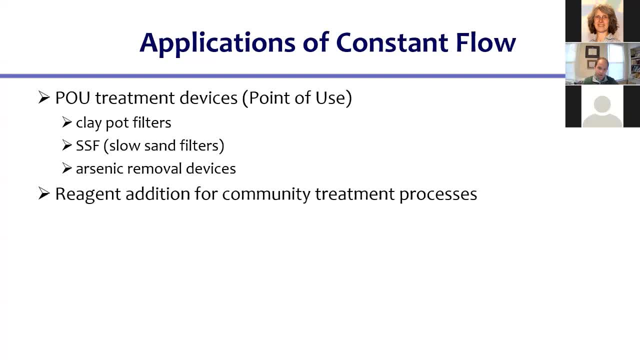 point of use treatment devices. Okay, let's see if we can name the process for the chemical here. So if you're adding alum or polyaluminum chloride, I think you guys have gotten this far. Which process would you guys guess here? 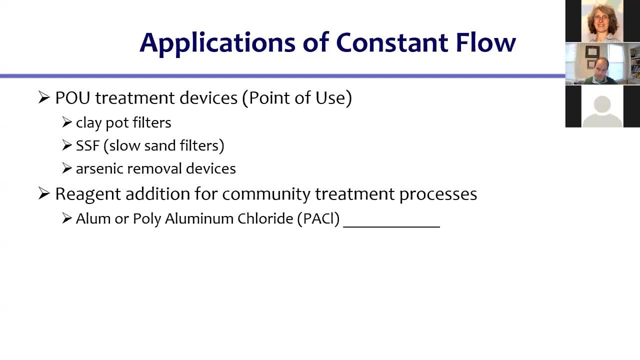 We got an answer in the chat: Coagulation Correct. Next, calcium or sodium hypochlorite. Got anyone who could talk in this, Those of you in 480.. 480.. You've had a lab where we Oh. 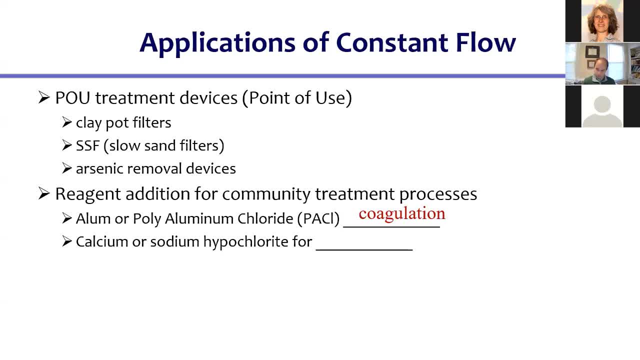 Don't make me cry. So hypochlorite would be a clue When you're using chlorine, that would be for disinfection. Like the lab that Dr Mastin was telling me about Sounds like quite the experiment. Is this whole class in 480?? 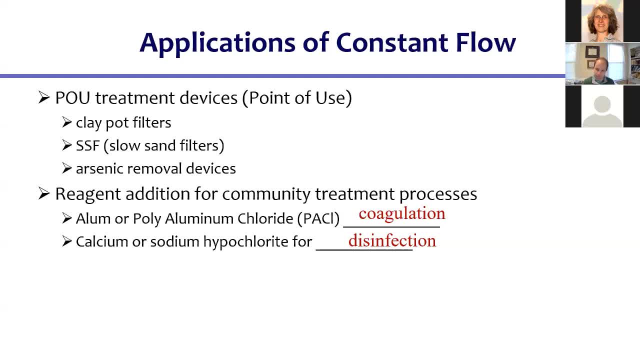 No, this is subset in both classes. Okay, So is that required for environmental but not for civil, or something Correct? Okay, And then sodium carbonate. I think you guys have also gotten to this part. Yes, they have. They've got a homework on it. 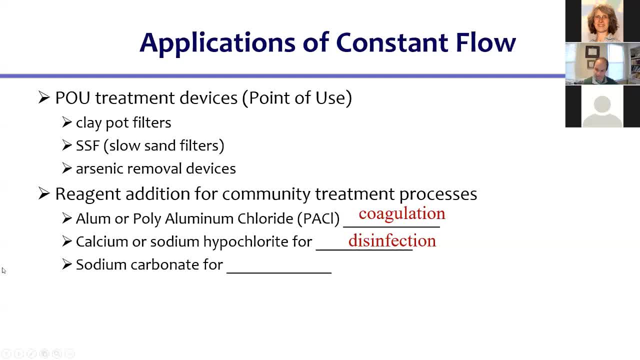 Any guesses? It's a clue. You've got a homework on it. We've got a softening question mark. Yeah, So softening pH control, Correct. So constant flow is desirable for treatment plans for optimal, For your processes to be optimal. 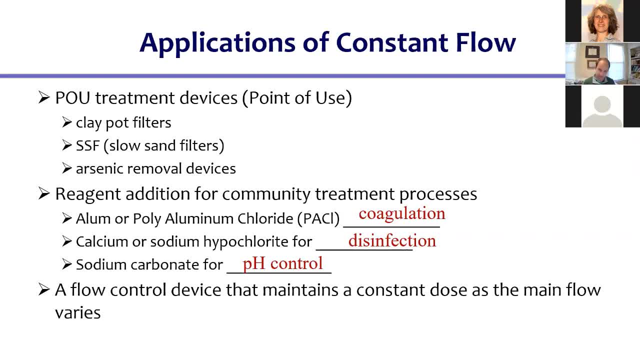 But it's not always the case where you have constant flow. In water treatment plants, conventionally you will have a constant flow because a lot of them are batch plants, Whereas wastewater treatment plants are variable, continuous flow that just run pretty much 24-7 and need to be designed for you know, various flow conditions, especially when you have combined. 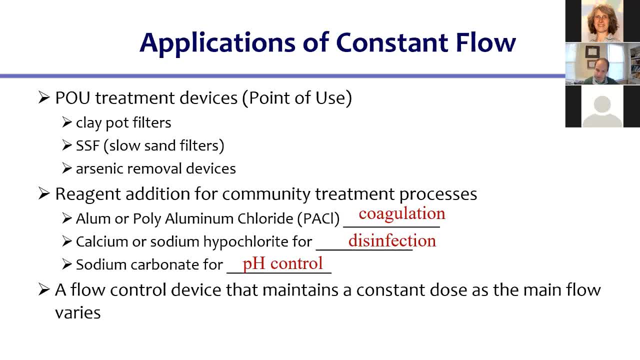 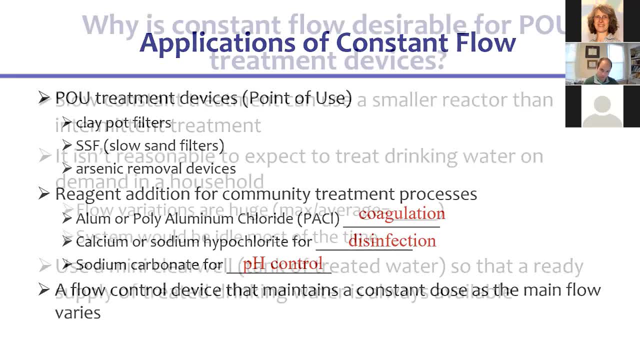 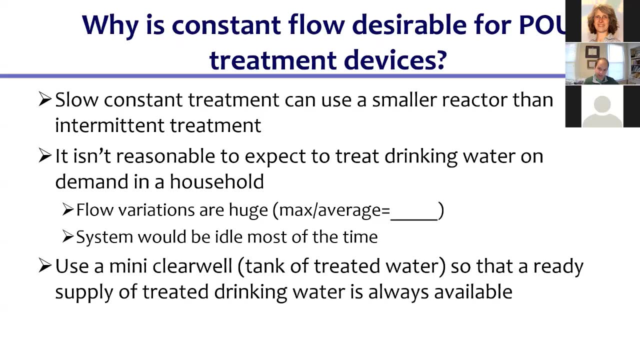 I mean a lot of communities still have combined sewer over time. I mean a lot of communities still have combined sewer over flows where storm events affect the flow coming in. So why is constant flow desirable? for point of use treatment, You can use a smaller reactor than intermittent treatment. 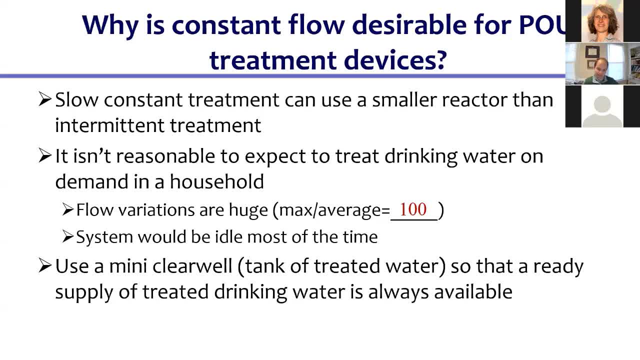 Flow variations are huge. This is more based on Agua Clara's mission, But it's not always the case for small communities that are used to walking to a well supply and filling up a bucket And now I mean are having basically a municipal supply. 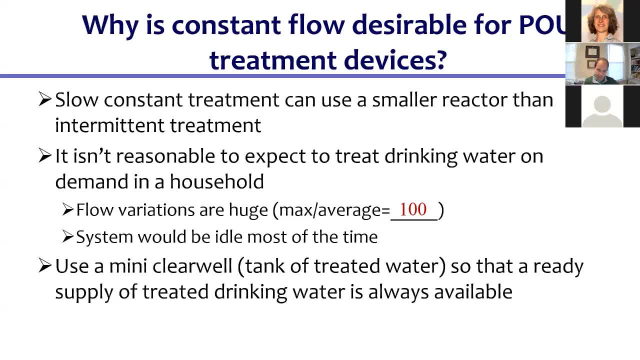 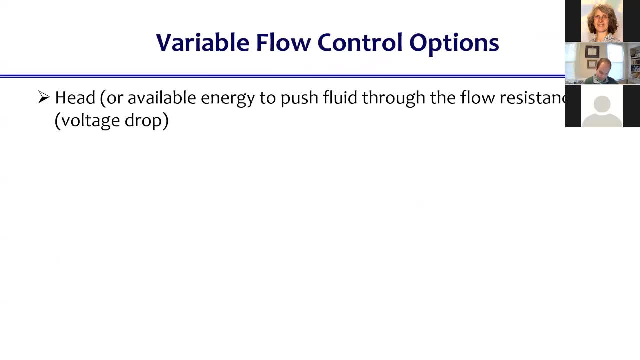 But the use of a tank of treated water supply. that, you know, is seen in conventional storage and distribution systems, Variable flow control options. So I like this slide because it uses metaphors with electrical systems And it's really interesting. It's really interesting. 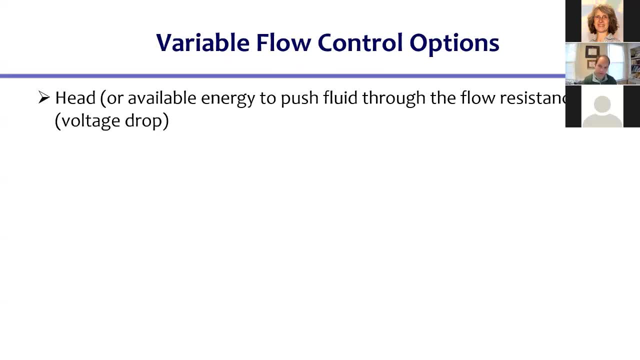 You can think of your head or the energy to push the fluid through as your voltage, And then your flow controls as resistors. Some examples of those: Orifice or any type of restriction, flow restriction, contraction. You can use porous media. 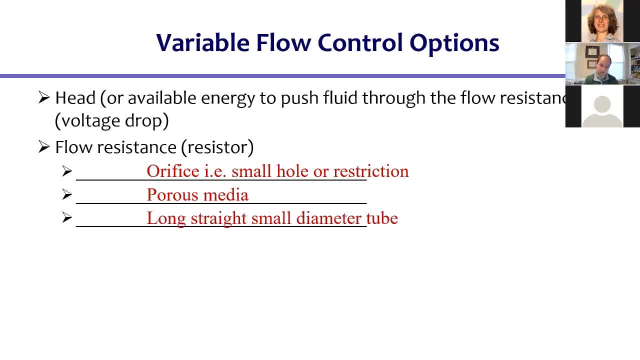 Like in a filter, or long, straight, small diameter tube, which is very common in Agua Clara applications, And then they're either the head or the resistance to vary the flow rate And the flow rate they are calling the current, for you know the electrical metaphor. 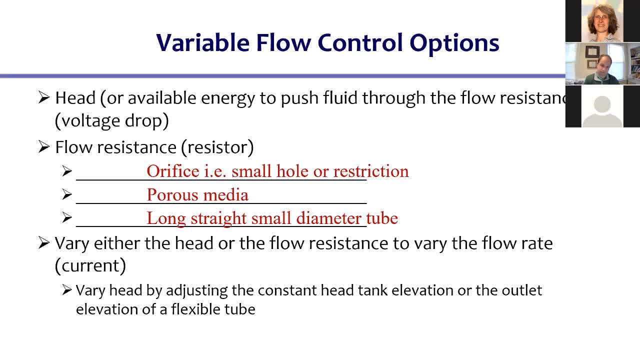 And you can vary head by adjusting the constant, the inlet or outlet elevation, Or by adjusting a valve, which in conventional treatment you see a lot more valves than at Agua Clara, But we do still use valves in both. So that was, you could see that whole. I still reference those slides a lot when I want to think about flow control. 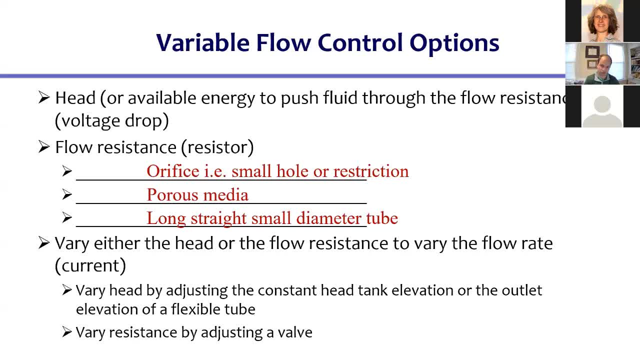 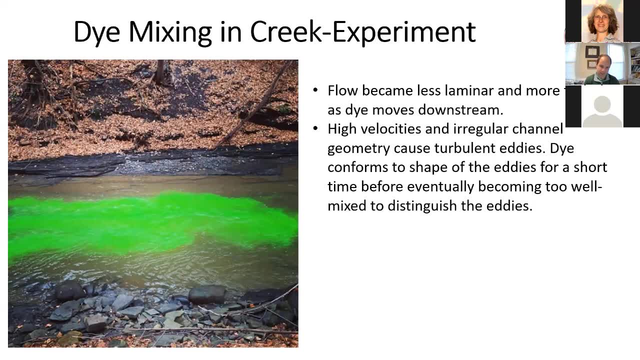 And I encourage you to download the PowerPoint. Here's another slide. Here's another cool experiment I did in grad school. We- I got a good photo of it too- We put in dye, probably about 30 yards upstream from where I took the photo. 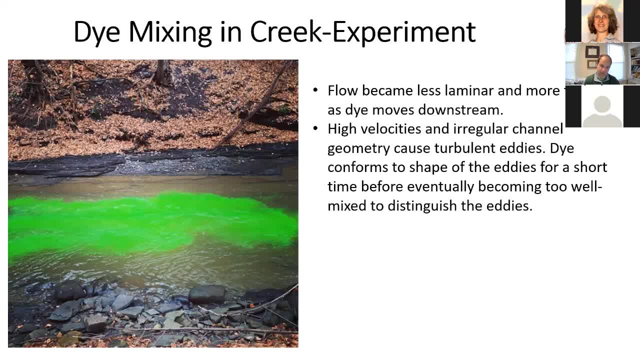 And observed the mixing patterns and profile. So, as we became, as we moved more downstream, the flow became less laminar and more turbulent Due to high velocities and irregular channel geometry, causing turbulent eddies, And the dye conforms to the shape of the eddies for a short time. 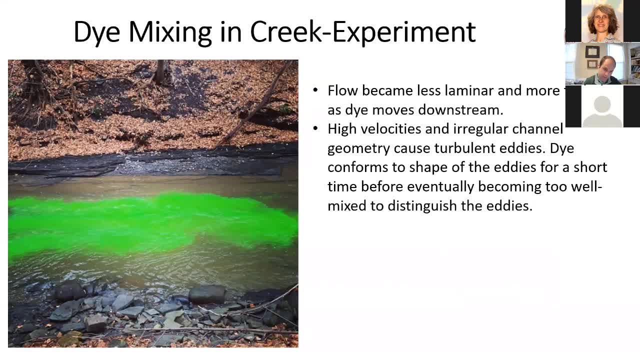 As I think you can kind of see in some little spots. But eventually, basically right after this, it becomes too well mixed to distinguish the eddies And it's just kind of well mixed, Kind of a well mixed solution- moving down the river turbulently. 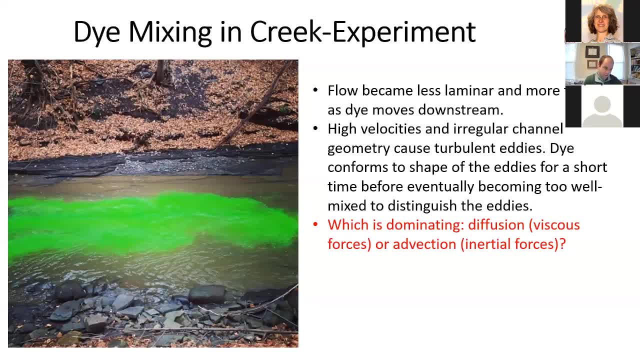 So quiz which is dominating diffusion, or aka viscous forces or advection inertial forces? Anyone have an idea? This doesn't have much to do with water and wastewater treatment. I just wanted to mix it in. This answer would be advection inertial forces. 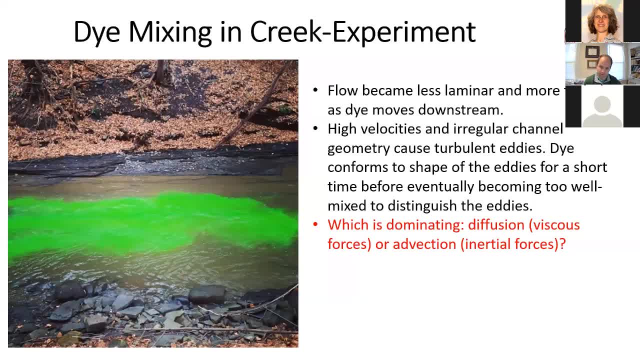 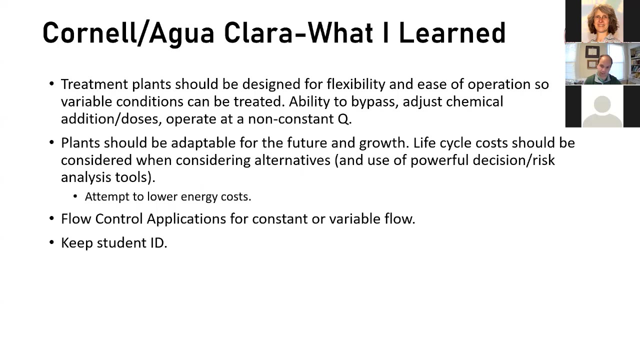 Once you leave laminar flow and you have turbulent flow, your inertia or momentum is going to dominate, rather than viscous forces or molecular diffusion having any impact on the fluid. So what did I learn? So these only need leadership. I will see if I get the needed stuff. 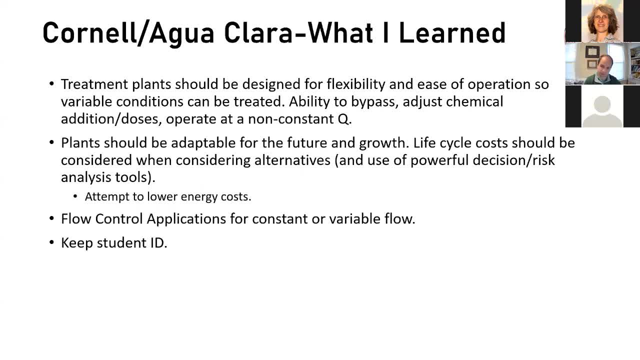 Uh, hissing. Well, I will let you touching me a little while, but you tell me just what you want. All right, thank you for all the very input And just make sure everyone is comfortable. just celebrate You guys getting the gets on. 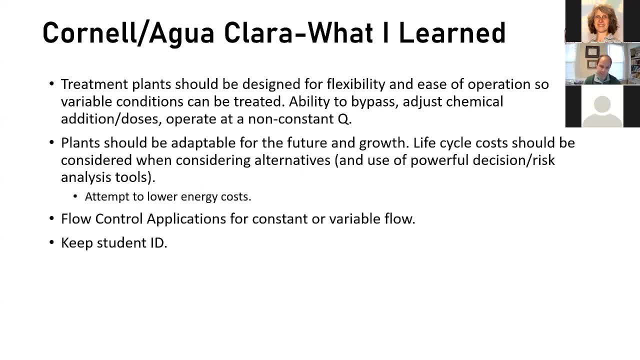 And then, when the next question comes up, There's somebody returning to the room. today, No problem is also important in a lot of our conventional work, our retrofits, So it's important to consider that. That's my next point. Future growth: lifecycle costs should be considered. 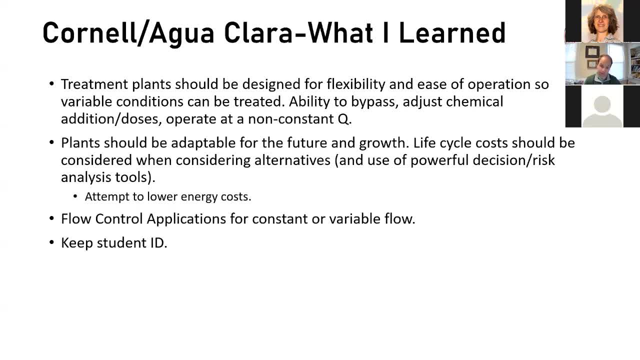 when considering alternatives. So Cornell is able to take decision analysis and risk analysis which, when considering alternatives or doing any type of cost benefit analysis, are just very powerful statistical tools. I actually- I'll show you something on that later- And the attempt to lower energy costs. 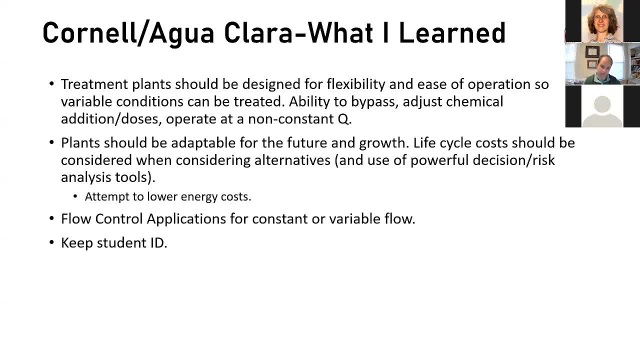 because obviously we were using 100% gravity plants, So I try to bring that into conventional plants when we think about that. I think I remember on one of the first days of the lecture- it was seven years ago, but Dr Mastin- 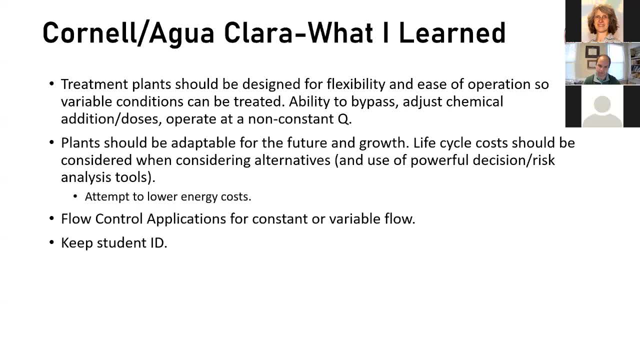 did your dad operate a treatment plant? What Where they- Sorry, What's that Finish? I think they were able to reuse the methane somehow, to reuse the energy. Yeah, so my dad was an electrician at a wastewater treatment plant. 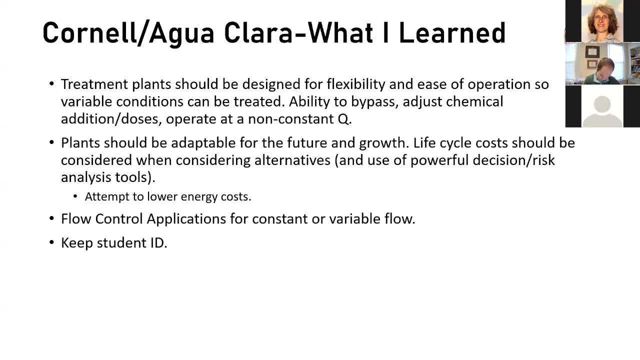 And they captured the methane from the digesters. They actually sold some of the excess methane to PSENG, which is public service energy and gas, and used the methane to heat the digesters, power the blowers for the aeration system. 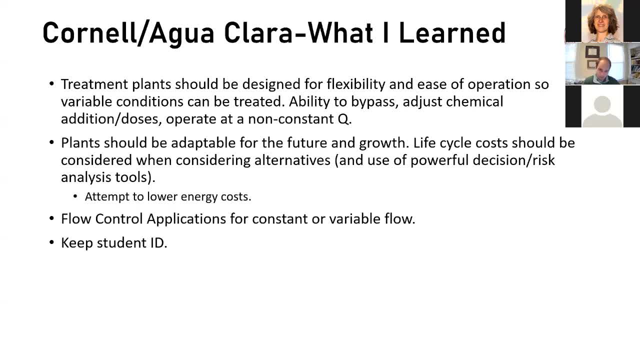 and heat some of the buildings. So, yeah, that's awesome, And that was way back in the day And you're seeing a lot of this now. And here's some stats: 33% of typical US energy budgets are vacated to water and wastewater treatment. 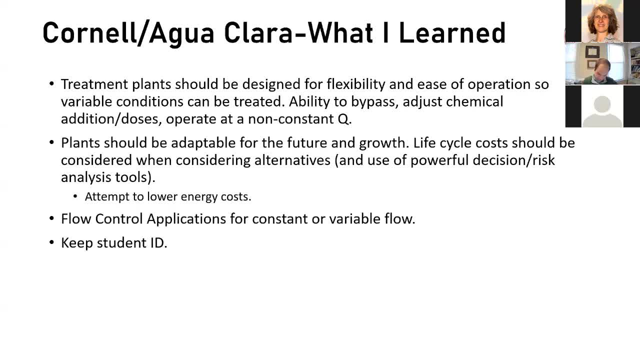 facilities- 3% to 4% of energy use in the United States, including 19% of California's used at water and wastewater treatment facilities, And not even the whole country has access to these facilities. so any way you can, 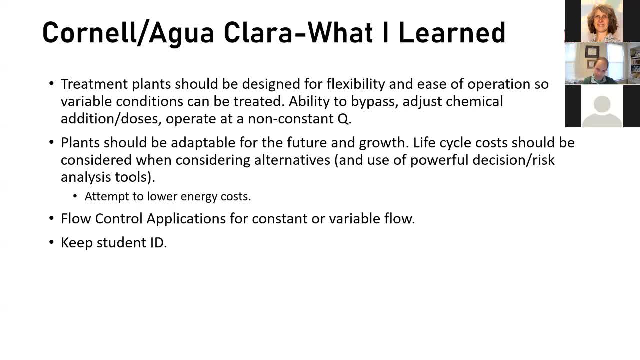 re-use, like Dr Madison's father did, or lower energy costs by using hydraulic gravity-powered processes rather than pumped or electrical. that's a plus, And when considering lifecycle costs it's a big plus. Flow control applications for constant or variable flow kind. 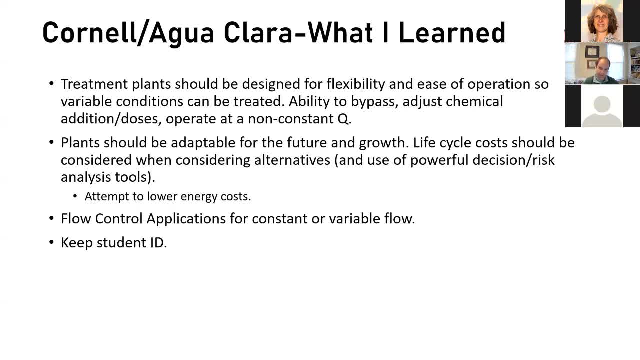 of. I kind of showed that on those three Agua Clara slides. I learned a lot about that. And then one last pro tip is to keep your student ID. I lost my MSU one. My Cornell ID does not have a year on it. 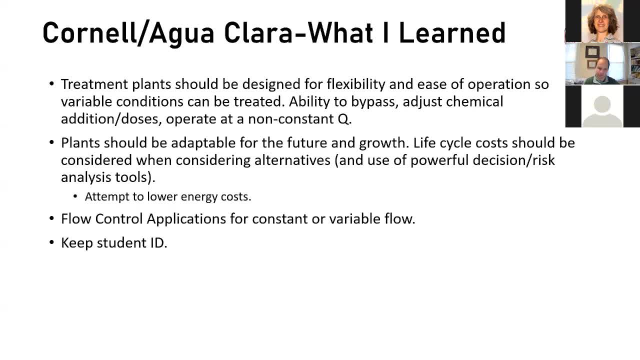 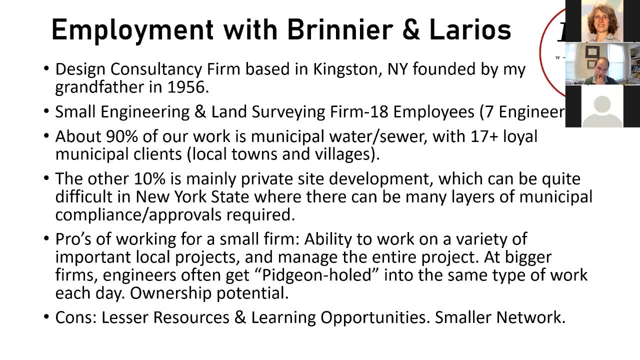 and I still am able to use it to get discount lift tickets at ski mountains and stuff like that. So just a little secret tip And that's about it for grad school. Then we move on to my employment. So I ended up turning down offers. from Arcadis and Hazen and Sawyer, who are two prestigious water design firms. I just didn't love the offers and the cost of living, And I also have a family business here in my hometown that my grandpa started in 1956. 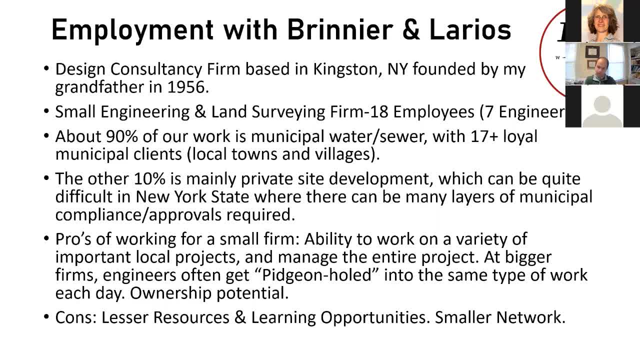 They're a small engineering and land surveying firm with seven engineers, now six PEs. We just hired a young project engineer, So I think it's the first time I'm not the youngest one in the office, which is nice, But we have about 90% of our work. 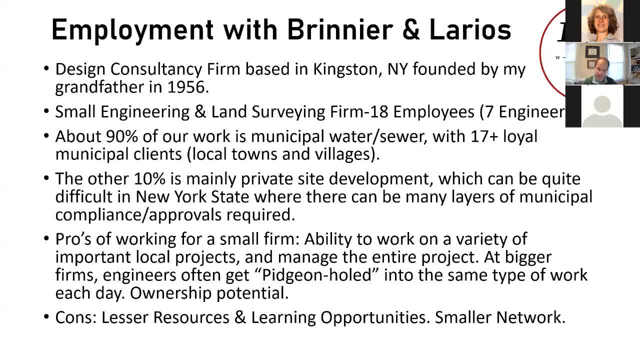 as municipal water and sewer. I think we have 17 or more loyal municipal clients, local towns and villages that have been coming to us, you know, since the 50s and trust us, and also we have all the survey, maps and records, past plans. so it's. 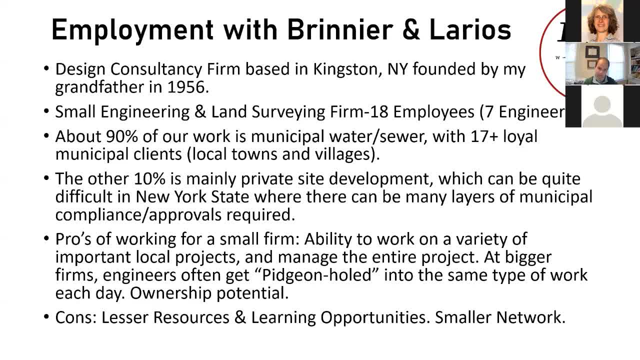 easier for them to have us do it, which is nice for us to have that. so we've worked right through COVID. we didn't have any remote municipal infrastructure was exempt and we are pretty isolated in our office. we have two big houses and between seven engineers and some admins we were pretty distant and there were no 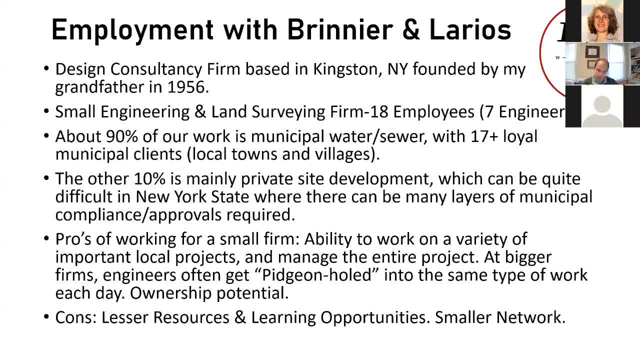 issues. it was actually quite busy construction wise this summer. so the other 10% of our work is mainly private site development, like guy design the car construction. and the other 10% of our work is mainly private site development, like guy design the car dealership last year, Dunkin Donuts. this can be quite difficult in New York. 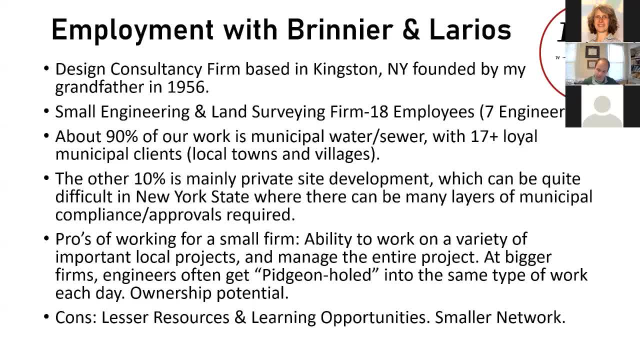 State. there's a lot of layers: municipal compliance and approvals required, zoning and planning boards, all kinds of historic landmark commissions and archaea, archaeological studies, endangered species- it's called a seeker review. state environment, state environmental quality review is often required. so we help our private site development clients get. 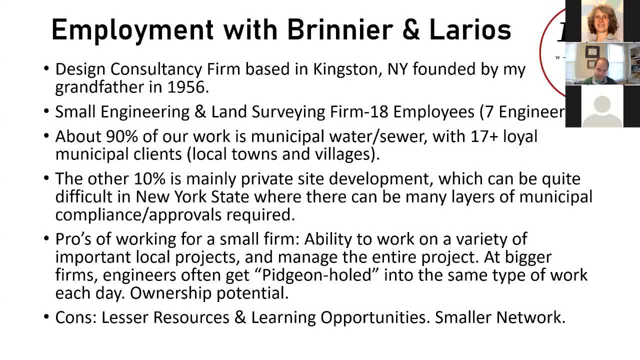 through the compliance process and get their permits, as well as developing plans that need to have a landscape plan, lighting plans that you know everything you can imagine. so some pros and cons of working for a small firm. I like, I like it. it gives you the ability to work on a variety of important local 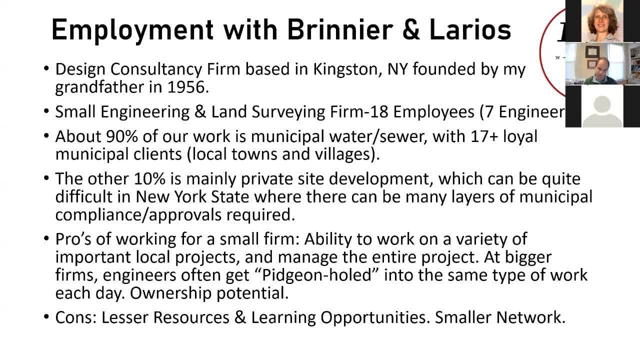 projects and manage the entire project. you still are working on a team, but um they uh like important local projects. i i'm working on our local hospitals being redesigned and you know it's rewarding when you get to see stuff like that come to fruition and you drive past and you can say how i did that, you know um. 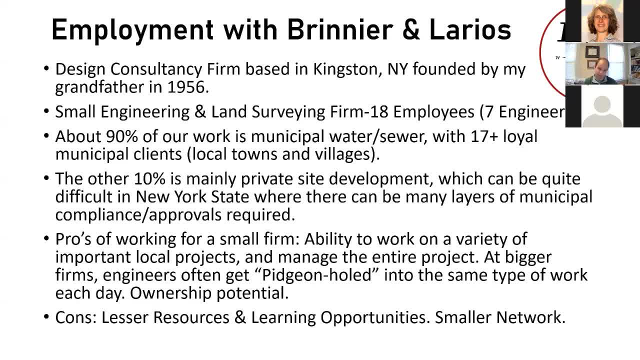 and also a bigger firm's. engineers often get pigeonholed, uh into the same type of work each day. where you know, i'll talk to some friends that are working the city, working long hours, and they're basically just running the same hydraulic model uh every day, maybe for a 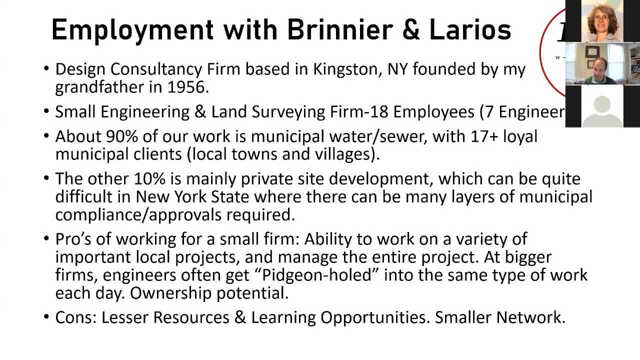 different project, but they are, you know, kind of in one role. whereas i do, i have the opportunity to work on site development and stormwater stuff, as well as water and wastewater and all kinds of different jobs. um, some cons. um, you are gonna have lesser resources and maybe lesser learning. 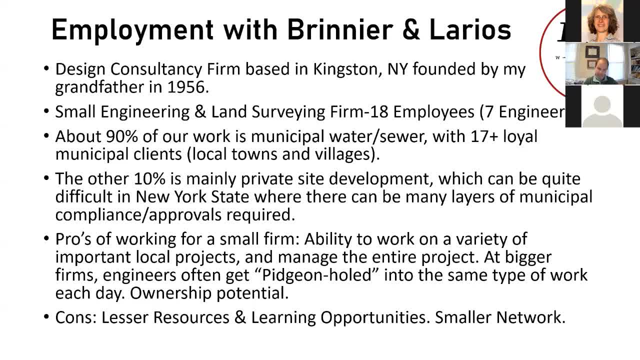 opportunities. some big firms will pay for you to go back to school at night if you want, um, and just have more staff, um, more you know, more resources, um, and you have a, you know, with smaller network at a small firm, obviously, um, and there's less competition, like, uh, i think i thrived in school because i always wanted to. 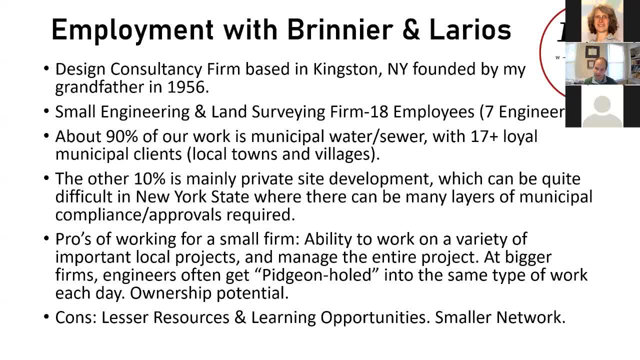 be towards, you know, the top of the class and, um, sometimes that's hurt me here, where, um, i'm not at a firm with a bunch of contemporaries competing with me, i'm, you know, the other professional engineers of this firm are. have been here since the 70s and 80s. 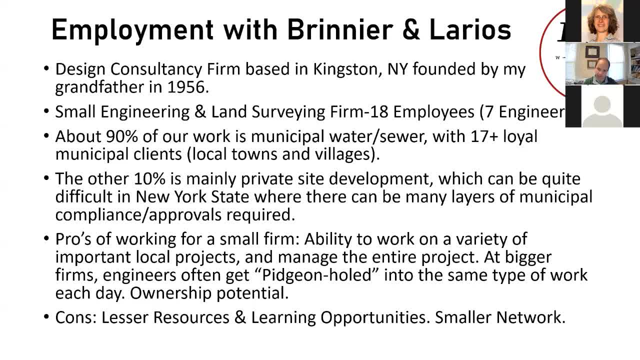 and um. so i was always the project engineer to their senior project engineer and i mean, i kind of just thrived on competition, but that's me personally. um, there's definitely pros and cons, but uh, again, this is my, my bias. i prefer this small, small firm feel. 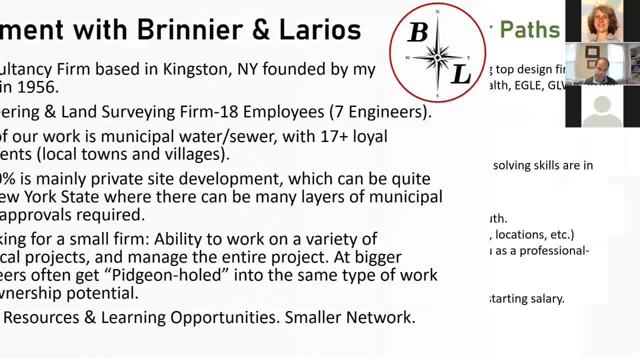 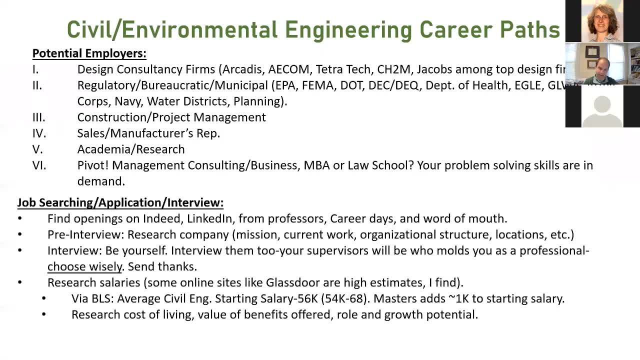 especially from around, uh, the eighties down south. you know they don't have anything but a lot of um considering. I'm kind of a legacy. So here are some career paths, basically all the career paths you could take. So I would be under number one design consultancy firm. I list some of the top. 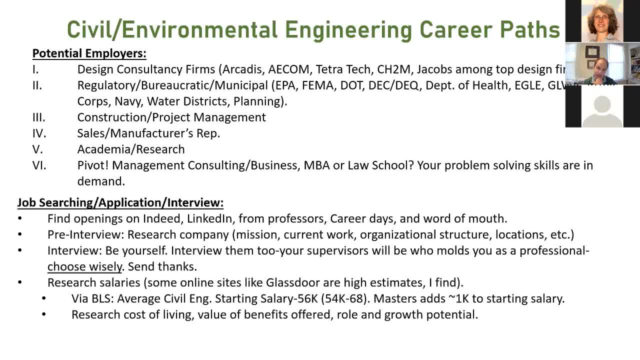 ones there. Regulatory, bureaucratic, municipal- a ton of jobs in this area available. I recently was looking at job openings. Seems that almost every federal department- the Army, Navy, the Department of Interior- is looking for environmental engineers, water districts and planning. And then 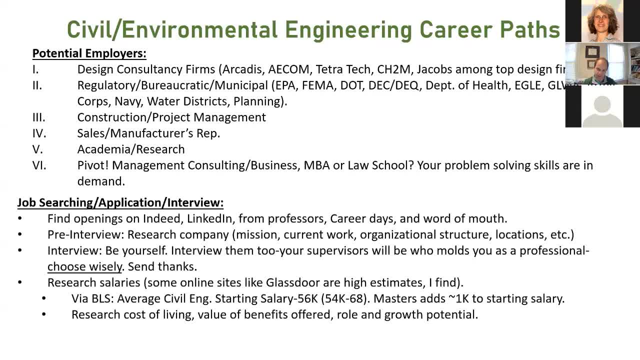 I think I saw some in Michigan for Great Lakes Water Association and DEQ. We have the DEC here. you guys guys call it the EQ, but those jobs typically have great benefits and are not as demanding as a design consultant's job, Construction project management. so we do a good amount of this too. but there are firms 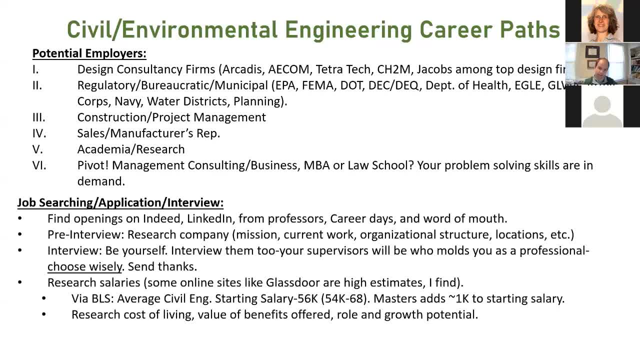 that just do construction and project management and there seems to be a lot of money in that area. You can work in sales as a manufacturer's rep, so you would come and try to pitch your product to a design engineer like us for us to spec in our designs. 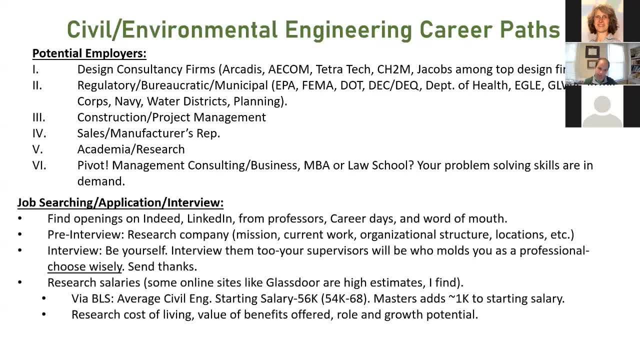 So we have people all the time come with their you know, trying to show us their new pipes and pumps and all kinds of stormwater solutions. That type of job is really all about. you know how much you're able to sell commission-based. 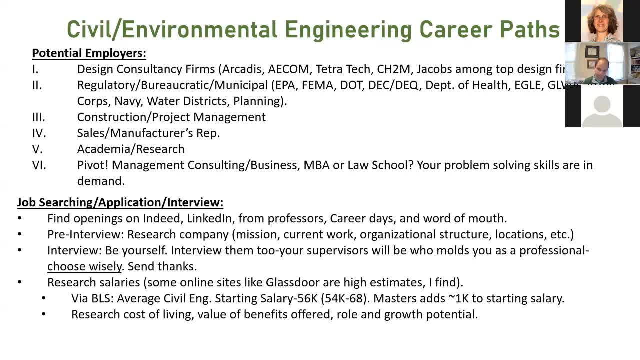 I'm sure Academics research, that would be a PhD path. Dr Mastin would be able to talk to any of you more about that. It seems like people are pretty happy in that field. I really wouldn't know. And then you can always pivot. 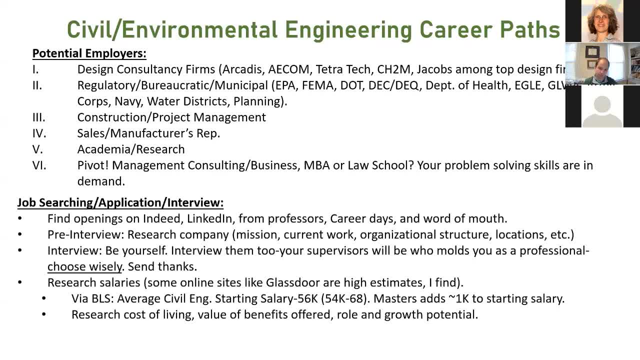 I saw a lot of Cornell grads from my master's program get jobs at prestigious management consulting firms, businesses. You can go for an MBA or go to law school As an engineer. your problem-solving skills are always going to be in demand is what I 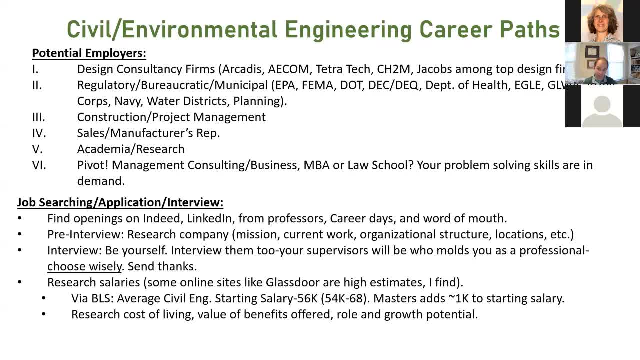 found, and they'll help you in other areas of your life too. As far as job searching applications, Interviewing, I find Indeed is the best for job listings, but LinkedIn has a lot too. You should all develop a LinkedIn profile because you apply for a job on LinkedIn, you're. 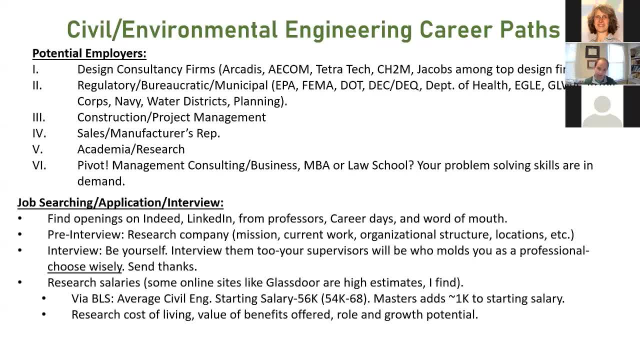 basically just applying with your profile. Professors will post jobs. Dr Mastin was nice enough to post a job opening we had here to you guys this spring. So yeah, Thank you. And word of mouth, which actually believe it or not, is how a lot of interviews get. 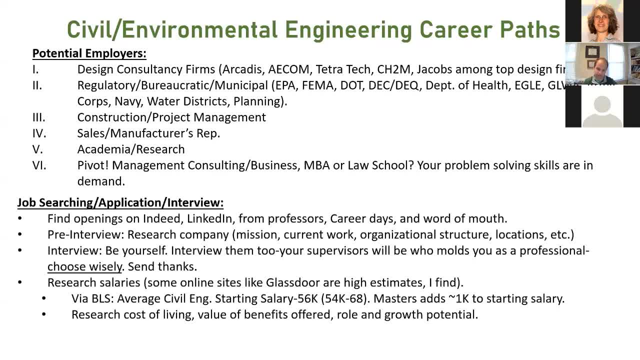 set up and how a lot of the most successful arrangements are made. Pre-interview, I would say it's important to research the company, their mission, current work, their structure, their locations. Be prepared to ask some questions. It's impressive to know that you've researched. 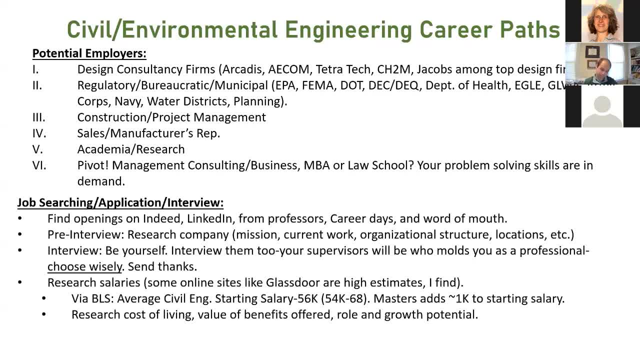 Yeah, I've researched them And as far as interviewing, I'd say: be yourself- I mean, you don't want to fake it or come off as anything else, I'd say- And interview them too. Your supervisors will be the people that mold you as a professional. 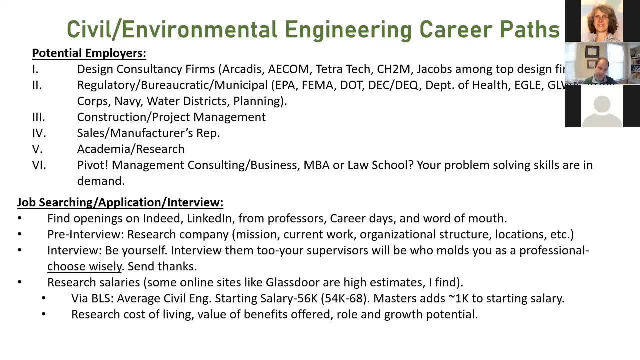 So it's important to choose wisely And after any interview just send thanks to anyone you met with And then you can do salary research. Bureau of Labor Statistics this year says the average civil engineer starts around 56K, ranging from 54 to 68.. 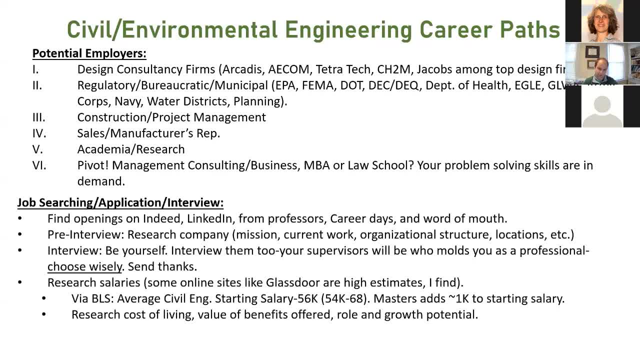 And they say a master's adds about $1,000 in starting salary And I think it's also important to research cost of living, the value of the benefits you're offered and what your role would be and how much growth potential there is at. 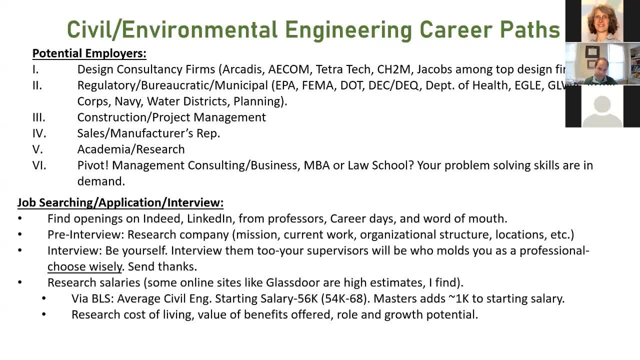 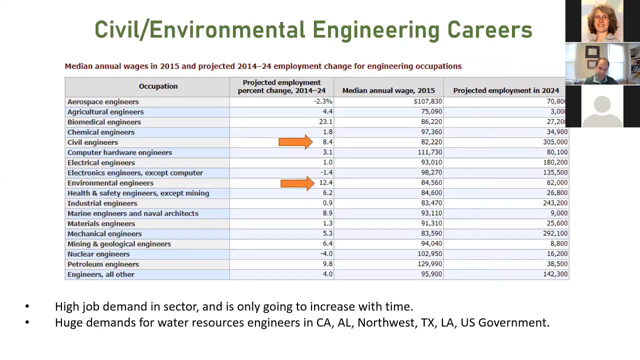 that firm- I can't stress it enough- To choose, To choose wisely in this regard and to interview them as a firm, because you don't want to go somewhere where you're not going to grow. So here's a chart projecting from 2014 to 2024, and just showing the huge demand for 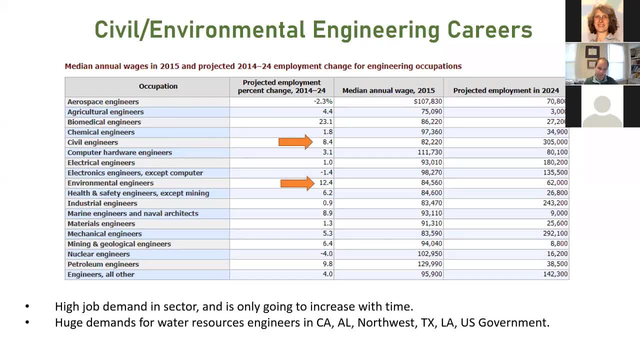 civil environmental engineers. Hopefully in the second column you would see the wages start to rise with the demand. It hasn't quite happened yet, But there's a huge demand in the sector and it's only going to increase with time because our infrastructure is ageing. 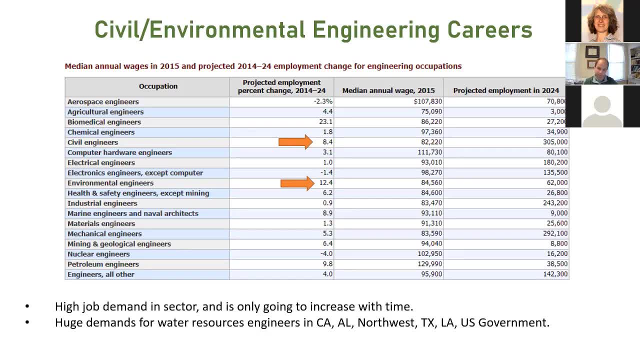 We're going to be, you know, retrofitting all of our- you know- 1970s treatment plants and our distribution systems. We're going to be going to reverse office. We're going to be doing all the things that we had to do. 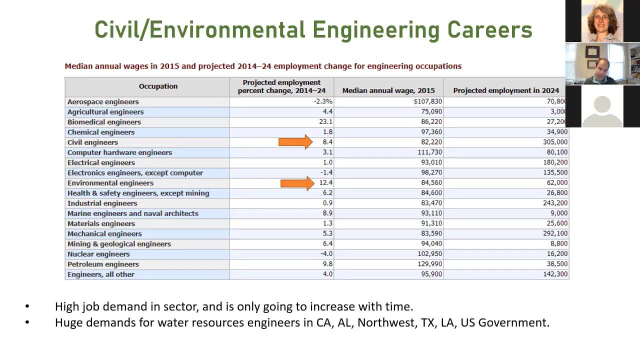 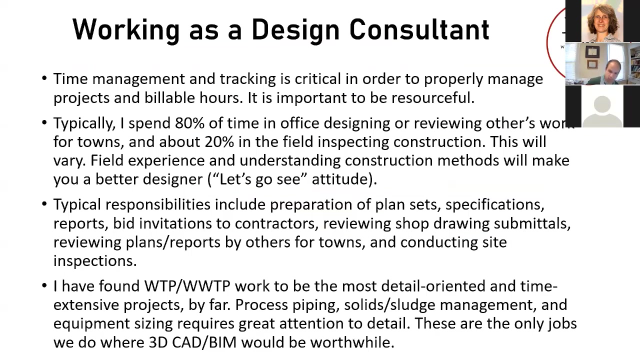 systems are much older than that. So I found, especially on the job search sites, California, Alaska, the Northwest Texas, Louisiana and US government positions all over the country are looking for you. So, as a design consultant, time management and tracking is critical in order to properly manage. 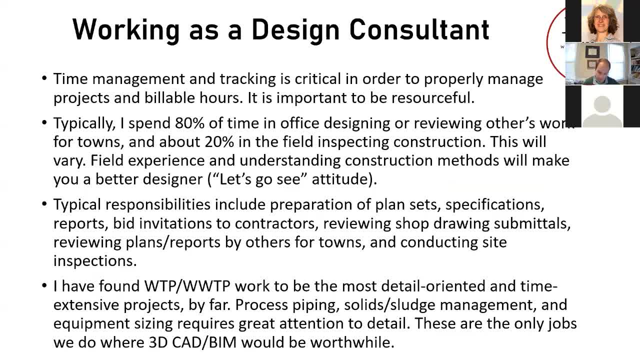 projects and billable hours and it's important to be resourceful. So this is the tough part of being a design consultant: billable hours. you can't really waste time or you don't get paid. you have to be billing hours clients, So that can be demanding at times as compared to maybe a 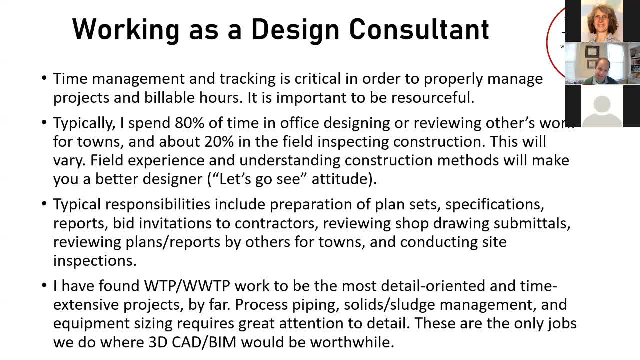 bureaucratic job. Typically my day to day, I spend about 80% of the time in the office designing And CAD or reviewing others work for towns or doing, you know, hydro, hydrological modeling or hydraulic modeling, and about 20% in the 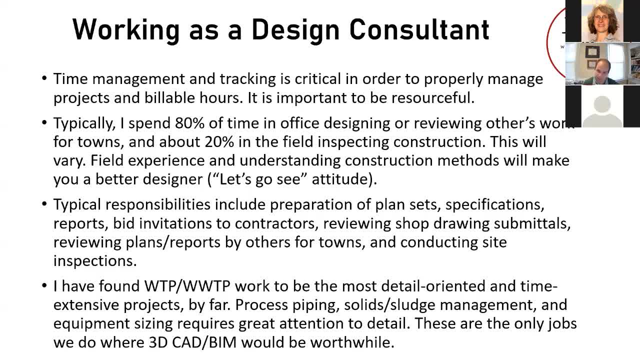 field inspecting construction on jobs that I have designed to make sure they're following the plans. 20%, maybe 25% in the summer, probably during COVID this summer, more like 30. Because it was such a good time to get stuff done with, with less traffic, everyone staying home. 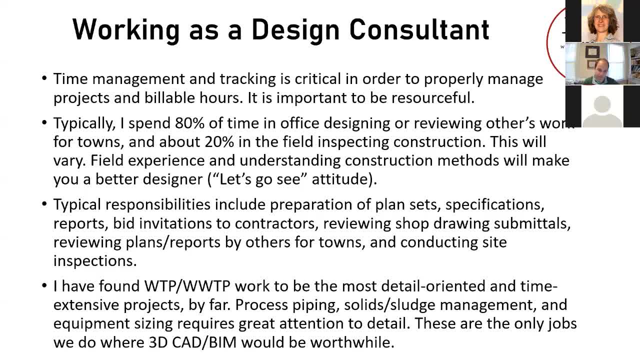 Field experience is crucial, and understanding construction methods will make you a better designer. Having a let's go see attitude is important, I think, even if you're designing a site from scratch and you want to go and just take a look at it outside, rather than a Google Earth aerial. 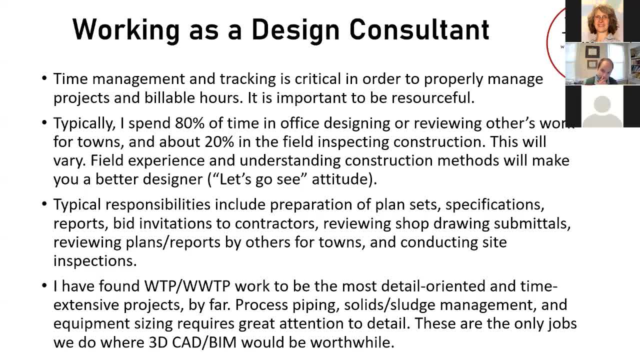 I think that's very important Typical responsibility responsibilities on typically preparing plan sets. I'll take you through a plan set later: Usually 15 to 20 sheets of AutoCAD specifications, reports, bid invitations to contractors, reviewing shop drawings, submittals from contractors for you know equipment and reviewing plans and reports done by others for towns that have us on retainer. 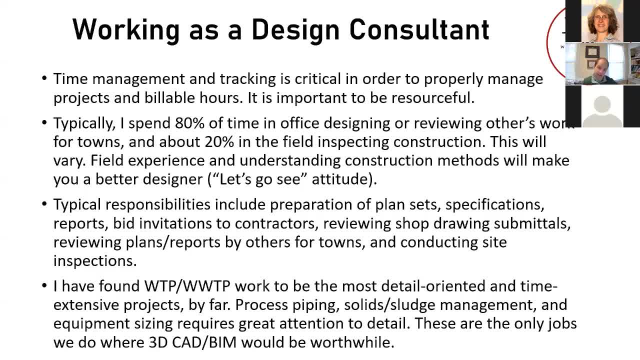 And conducting site inspections. So what I found is that water treatment work and wastewater treatment work Are by far the most detail oriented and time extensive. My opinion process. piping, solid sludge, management equipment, sizing- these all require great attention to detail And also, I'd say these are the only jobs where 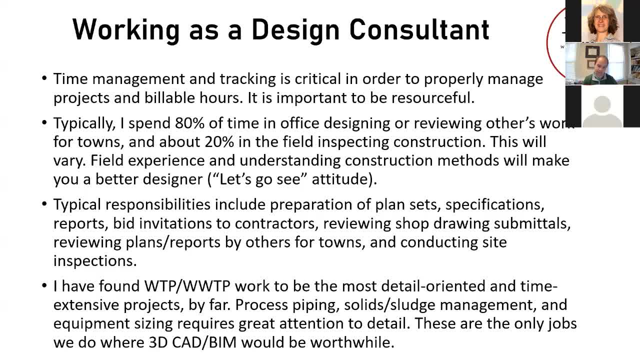 we would, And Right now we're 3D CAD and BIM would be worthwhile just to fit everything in a building's blueprint with the process piping and Everything. to avoid conflicts. We at our firm do not have any 3D CAD. I mean, we have civil CAD 3D, but all of our drafting is in 2D. 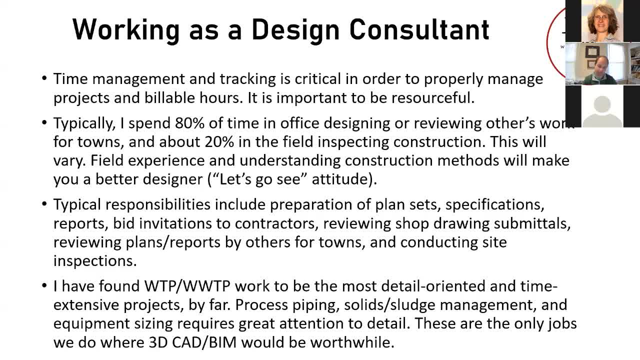 So if it got to be a huge treatment plant, we wouldn't bid on the job because our drafting capabilities are not there yet. We'll get there, I'm sure, but That's what I found. So that'd be a good skill to develop, and it's the BIM stuff. 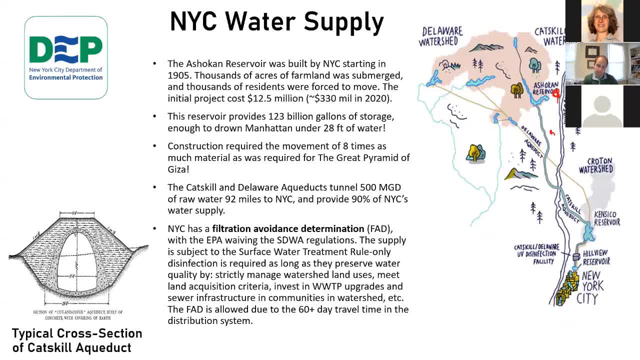 Alright. so if you remember the cover slide, I showed you the Ashokan Reservoir. I showed you the Ashokan Reservoir. I showed you the Ashokan Reservoir. Here I live in Kingston, which is, you know, just east of it on the Hudson, and village of New Palt is right in here. 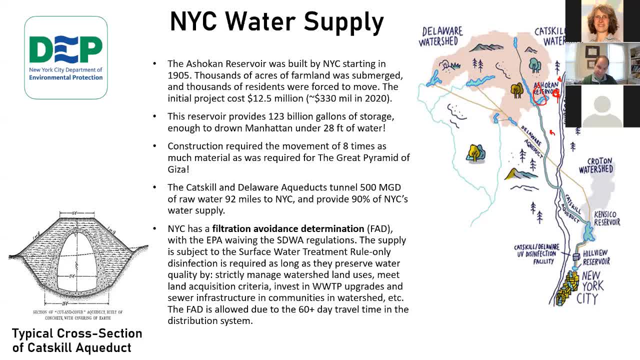 Near these aqueducts where you can see a cross section of the aqueduct. These have got to be the largest water transmission mains In the world, Just like an grilled Jake's tears. Oh, Of course They're Irregular and cross-section. but this one is 17 and a half feet, 17 onions shape, Some of its overground, Some of it's below. 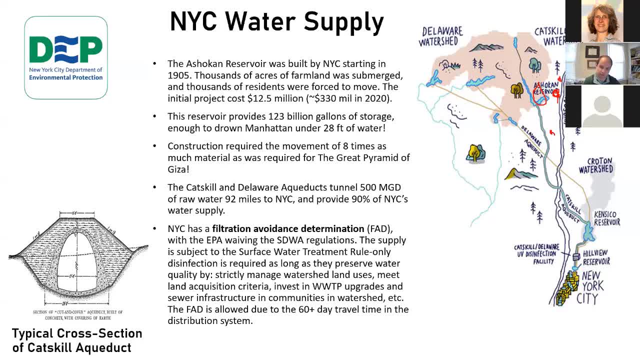 The Reservoir itself was built, The main Reservoir- million back then, which would be 330 million today. um, adjusting for inflation, enough uh storage to drown manhattan in 28 feet of water. the construction required the movement of eight times as much material as the great pyramid of giza, which is the largest of the pyramids. 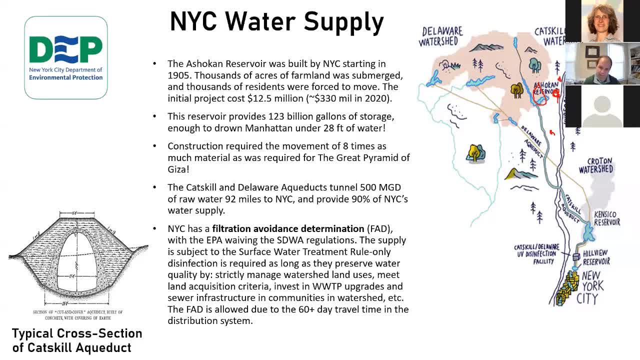 i thought that was a fun fact. um, these two aqueducts at delaware and the catskill uh tunnel 500 million gallons per day of raw water to new york city. uh, 92 miles from upstate where i live um and provide 90 of the city's water supply and the city has. 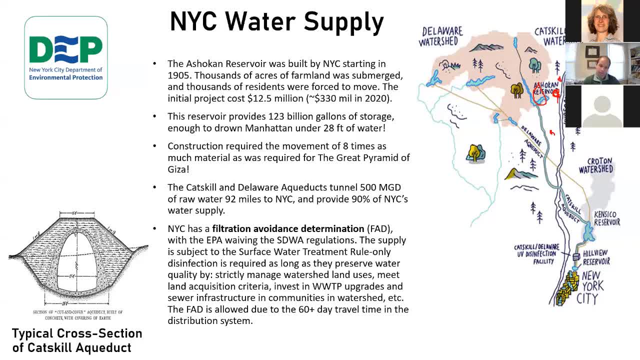 a filtration avoidance determination, meaning they don't have to filter like the surface war. um safe drinking water act would uh imply that's waived by the epa. there's a 60 plus day travel time in the distribution system. they still have to disinfect, which they do down here at a facility close to the city. um, they do have to do stuff in. 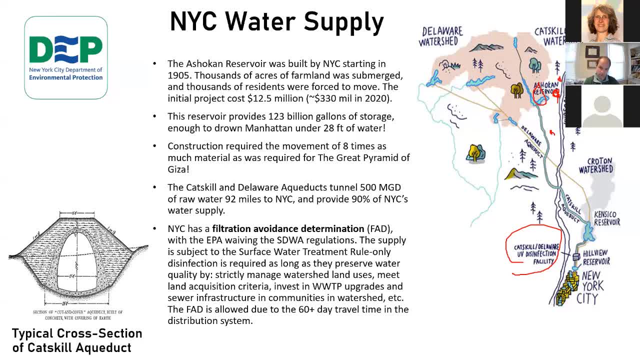 the watershed um, and invest in some of our local wastewater treatment plant upgrades and sewer infrastructure, uh, stuff like that, to keep this filtration avoidance um so. so two of the four jobs i'll talk about actually tap into these aqueducts. uh, raw water so, and the dep is the bureaucracy, um, in charge of the supply they seem to have. 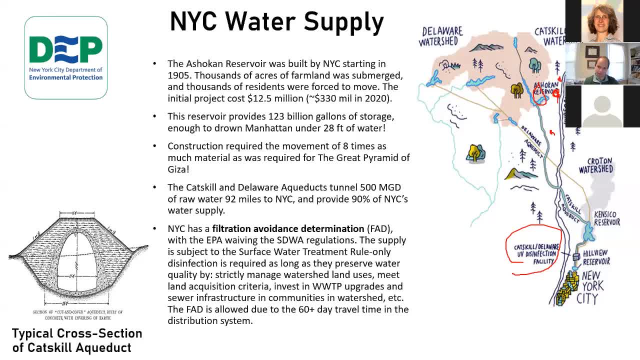 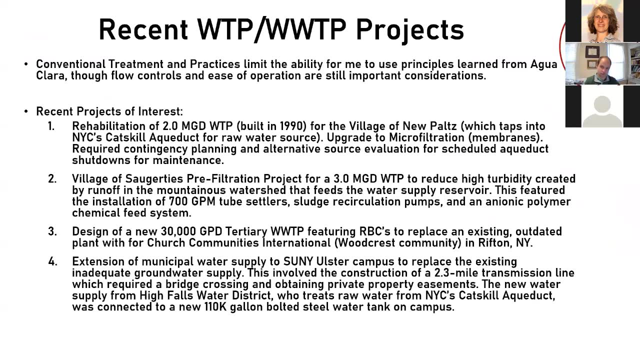 more power and better benefits than any other bureaucracy and, uh, we work with them a lot. they they're pretty good. so some recent water and wastewater treatment projects through veneer and larios that we've worked on um included village of new paltz two million gallon per day water treatment plant. um. 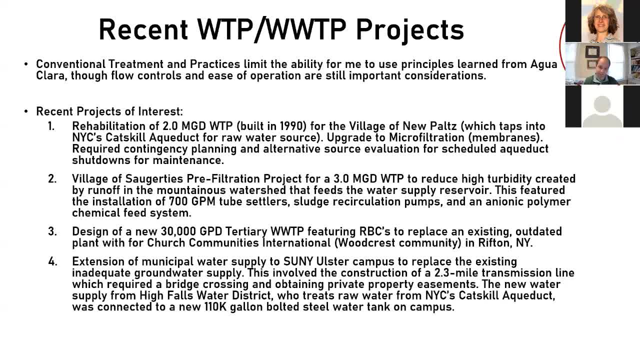 which taps into the casco aqueduct for the from the city um they upgraded from sand filters to membrane filtration, which i don't think you guys have gotten to yet. it's basically um pushing water at a high force through a semi-permeable membrane to remove. 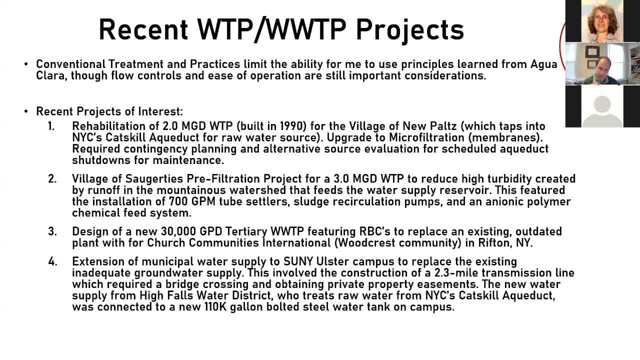 the smallest of contaminants, including, you know, giardia and all kinds of bacteria um. we use microfiltration in that one um and this one required contingency planning as the aqua ducts were shutting down for maintenance in for 60 years. so we're not going to. have to say the end of it yet. so just to add a quick note. responsible for that was: we're still going to work on it for a long time in the QA of 2020, because if we could provide those effects and those services that we can, we're hell in the house. 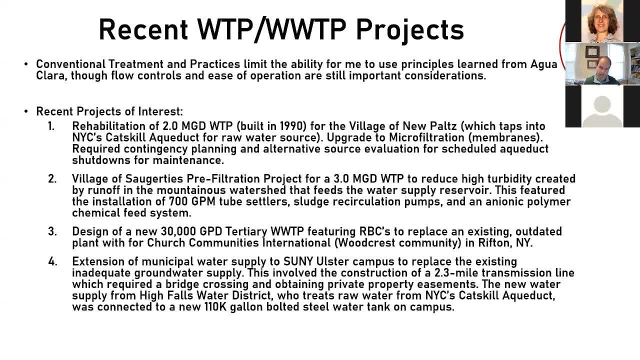 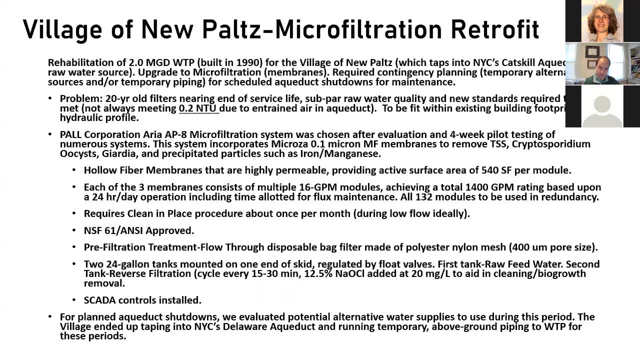 eight week periods for a couple of years. um, i actually did a report on cornell and decision analysis on that. um, let's see. i'll just get into the other projects as we get there. so in new paltz the problem was the 20 year old sand filters were nearing the end of their service life. 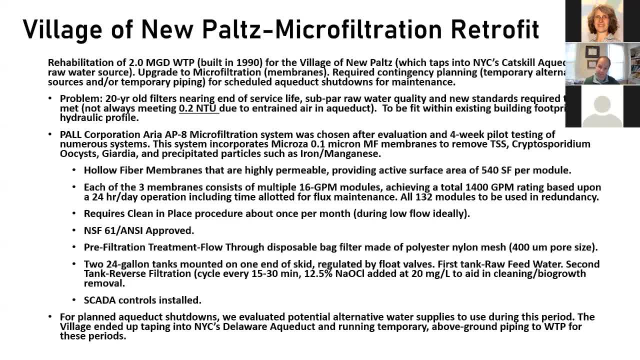 um, the raw water quality from the city's aqueduct was uh not great and uh, new standards required. uh 0.2 ntu. um, here's a quiz. uh, anyone know what ntu stands for? besides dr mastin, let's hear some spartan voices. 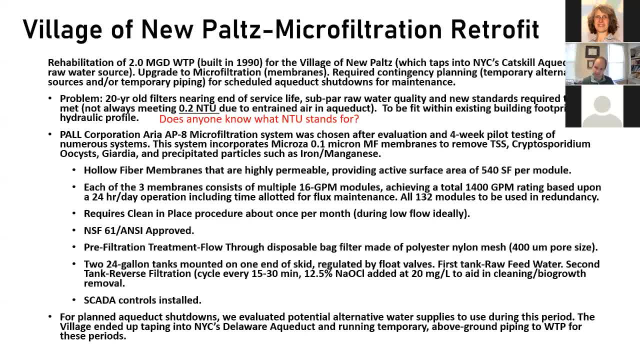 anybody here? no guesses. does it have to do with the turbidity? yes, so the last two are two turbidity unit and the n is going to be tough it. um is from the greek for cloudy, nephelometric um. i didn't think anyone would get it except dr maston um, actually even even dr. 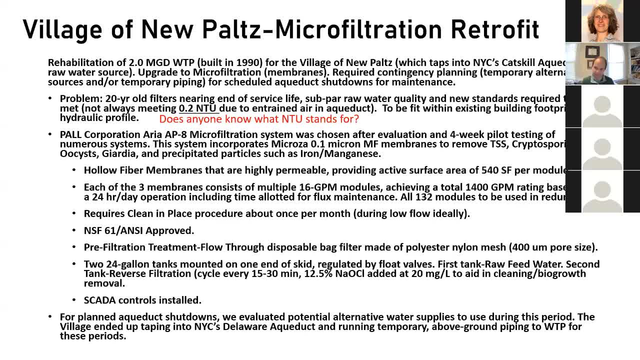 maston didn't know that it was the greek for cloudy. so i learned something- besides lots of other stuff that you've mentioned today, but i learned something new. i'm half greek, so i uh thought that was interesting: nephelometric greek for cloudy. so it's basically: yeah, turbidity, uh mud. 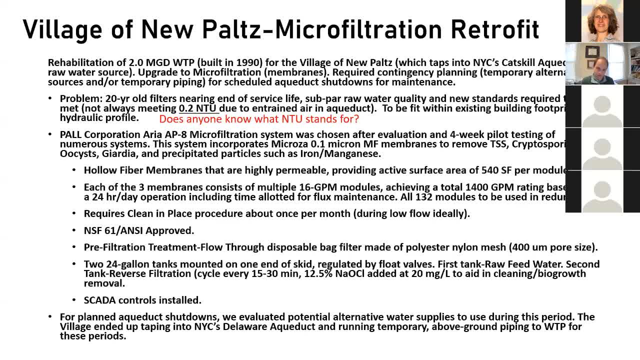 solids in your water. um so um, they use a paul paul, like my name- uh microfiltration system that was chosen after evaluating and doing a four-week pilot testing system as required by department of health. so when we're doing uh water treatment work, it's it's usually doh and uh wastewater treatment plant. 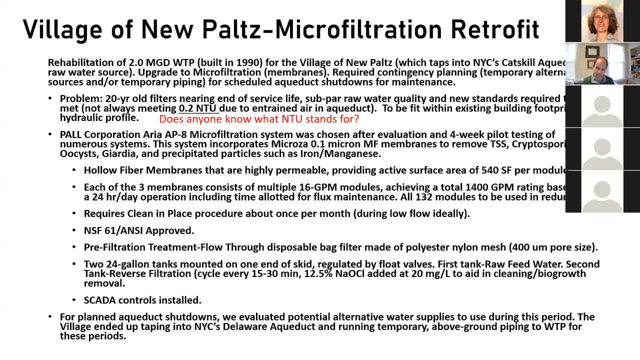 would be the dec department of health and the wastewater treatment plant would be the dc department of health, environmental conservation. So also NSF approval. it's important that any of the technology put in is improved, especially I mean it's required for municipal jobs. 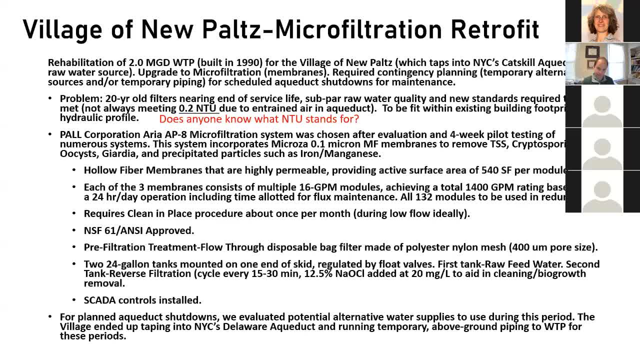 SCADA controls installed, for you know, real-time data and planned aqueducts required alternative source evaluation. I can get out of this presentation. How do I? If you go to share screen, yeah, and then you'll want to change your share screen from here to whatever you want the plan. 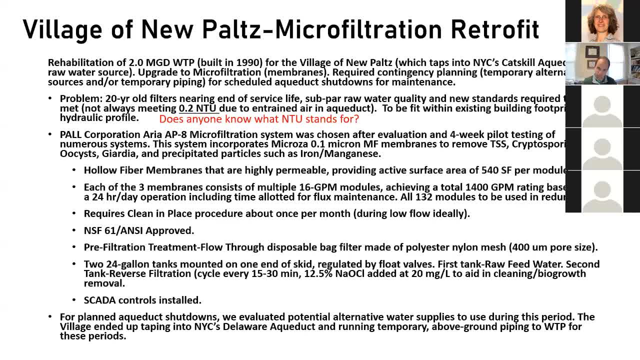 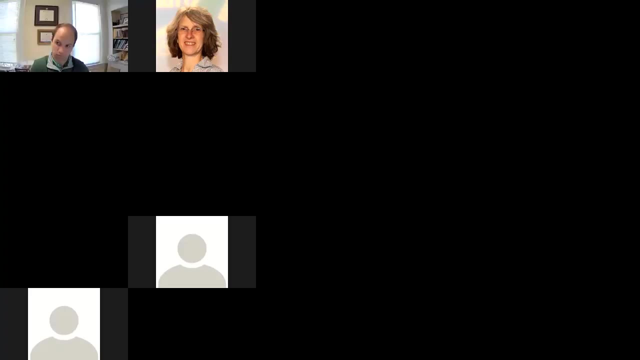 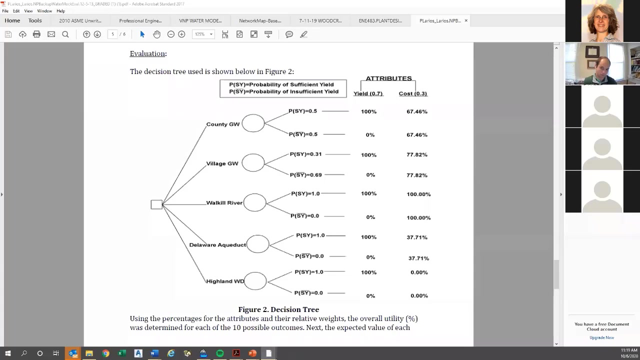 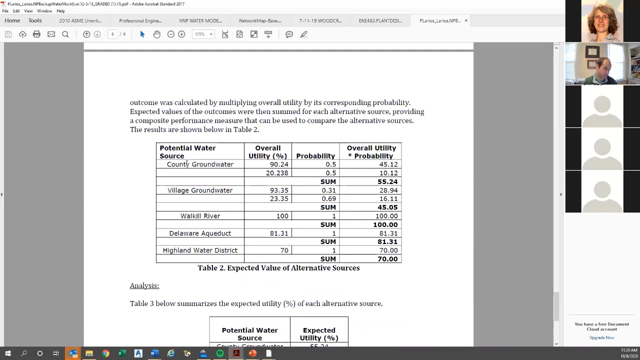 to be Okay. so at the bottom controls, where it says share screen, yep, and then i there. you should be able to go, and you yep, there you go. so you're showing the decision tree. now, paul, we can't, you're on mute now. 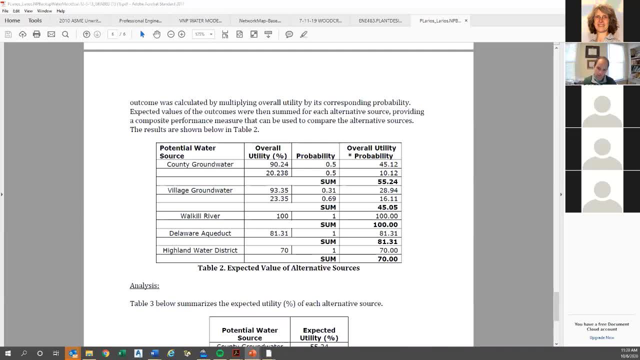 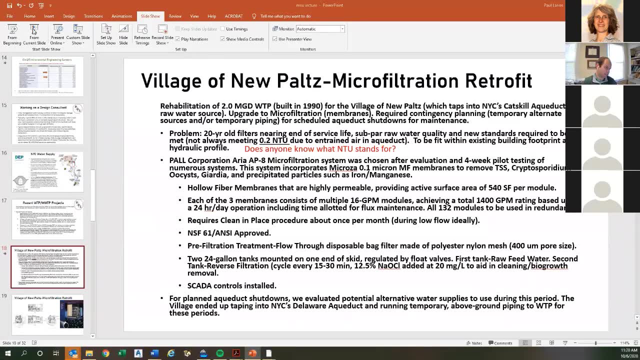 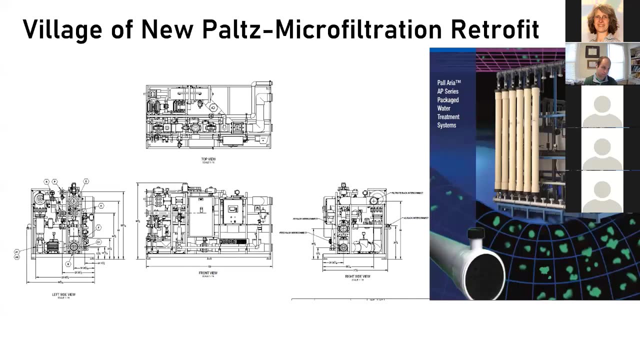 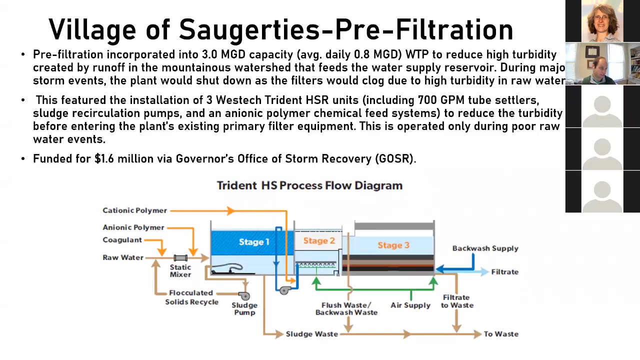 you got me now. now you're good, okay, so i just wanted to show some of the decision analysis stuff. so this is the microfiltration system, um, some some stuff from our plans and from the brochure, um, for new paltz, and then it's saugerties. um, we had three million gallon capacity, but the 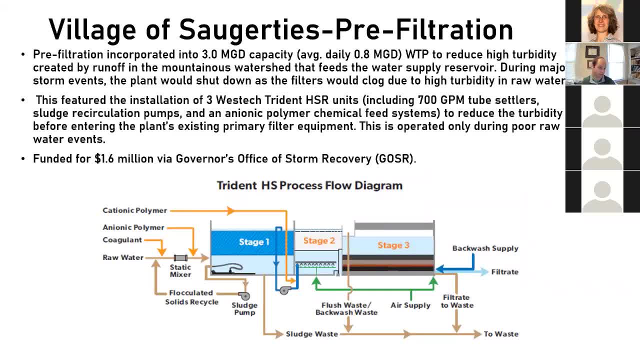 average daily is just 0.8 and the the goal here was to reduce high turbid. i mean you get storm events in a mountainous watershed and the water supply reservoir at you know, at the uh treatment plant site, is just um receiving really turbid water um, which can cause the filters you got to basically shut. 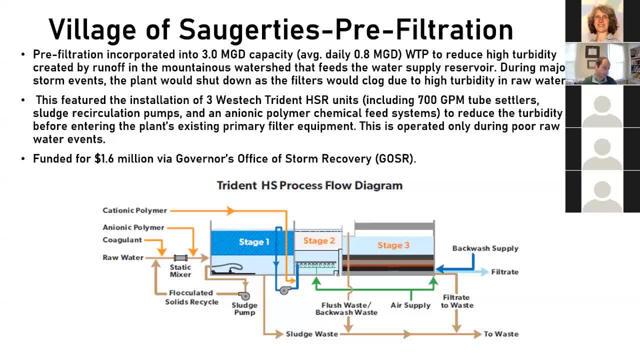 down the plant because the filters were clogging. so we put in a pre-filtration system that is actually normally bypassed except for during high storm events, and this included 700 gpm tube settlers, a whole feed chemical feed system so that coagulation. 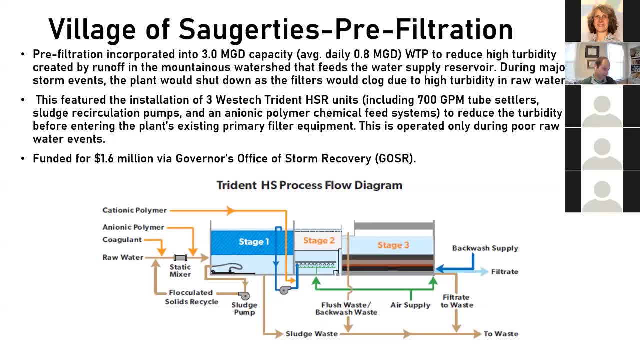 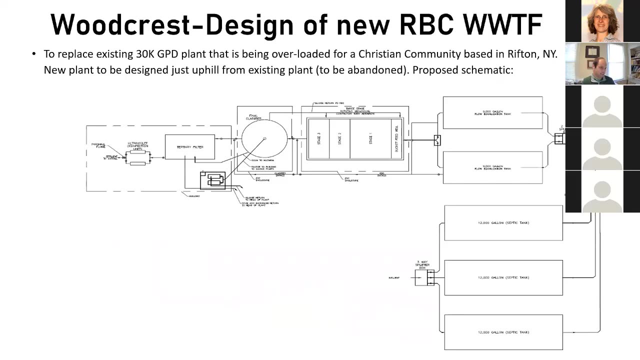 and mixing and everything can occur here and then go through. it still goes to the normal filtration and everything else in the plant after um and it's funded by gozer government office of storm recovery, which is a funding source here in new york. um, okay, woodcrest, this is a big private client of ours. it's a christian community. 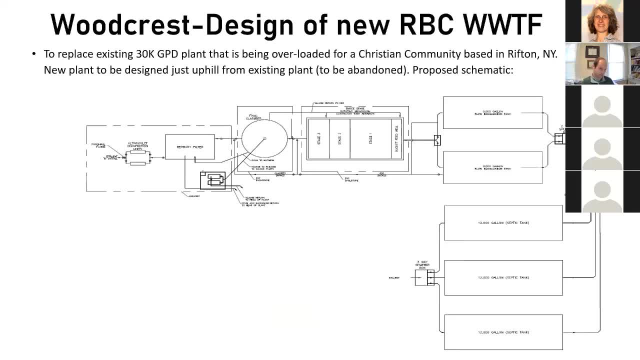 um, and here's a schematic: uh, it's actually the first one i designed. um, so this is an rbc plant: rotating biological contactors with aeration- um, pretty common for wastewater treatment, i'd say uh, nowadays, as opposed to like a trickling filter or something, um. so we started with septic tanks. 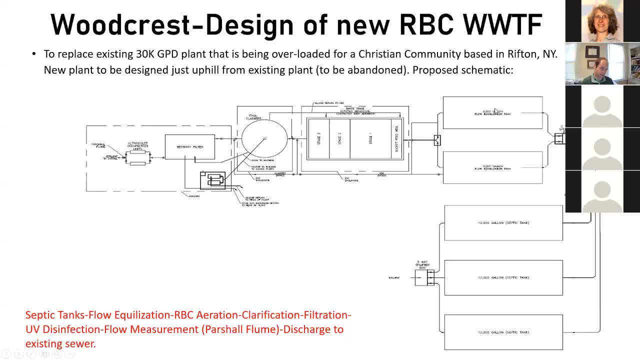 tanks and then flow equalization, which is huge, to you know, to get flow control, like I talked about in Agua Clara. We have these two 9,000 gallon tanks before the RBCs, multi-stage RBCs. to a clarifier, 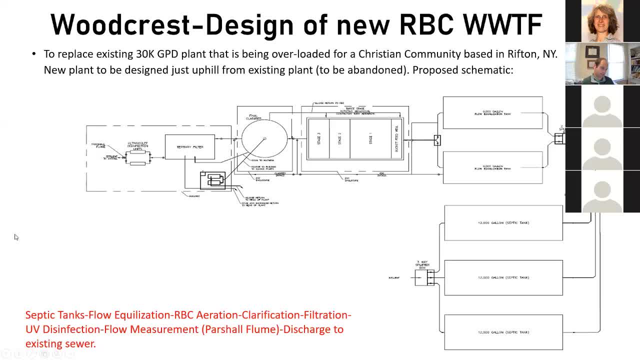 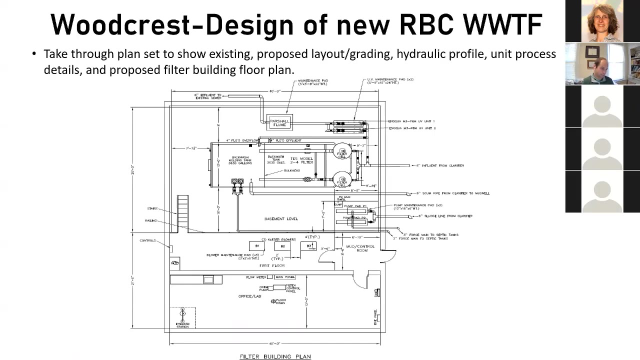 for settling. then scum and sludge go to pumps And there's a filter, UV disinfection, partial flume for flow measurement, and then there's a sewer line out to connect to an existing sewer. Here's the filtration building. 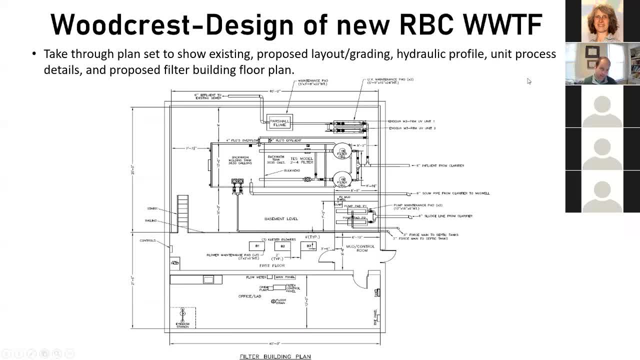 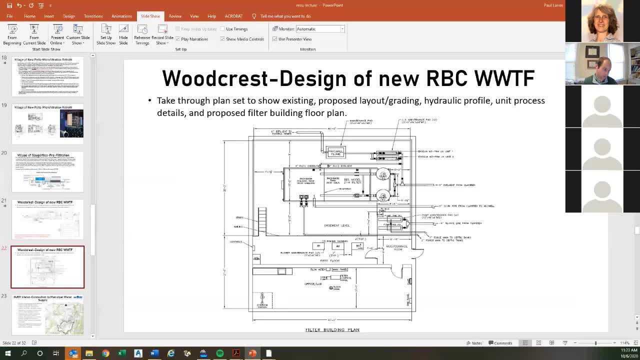 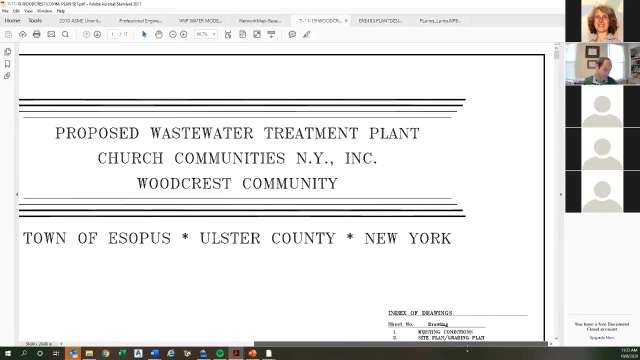 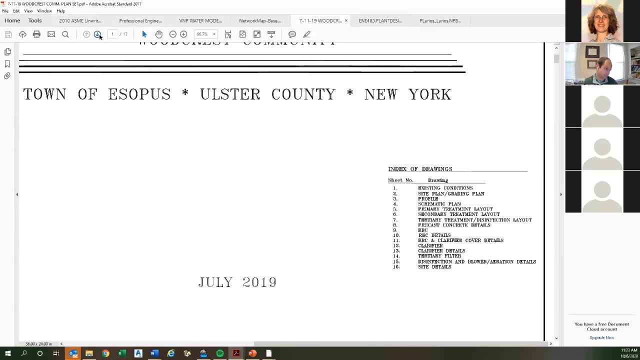 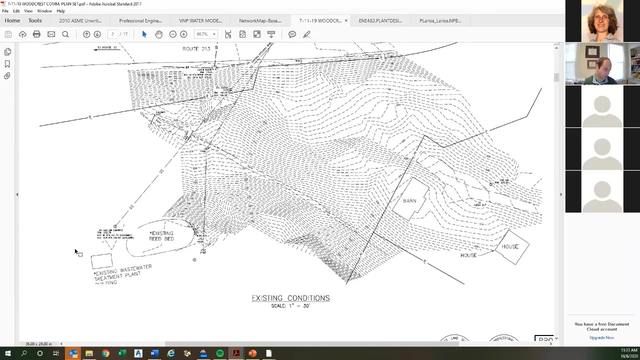 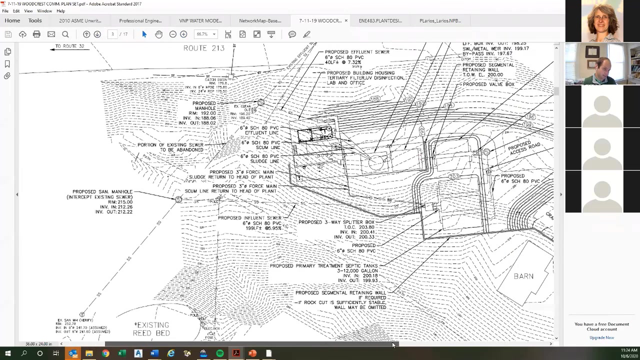 So I was going to take through some plans on this. Okay, So some typical plan set. There's our 16 sheets, so you always show existing conditions. Their existing plant was down here and was just overloaded and outdated, So here is the proposed plant. 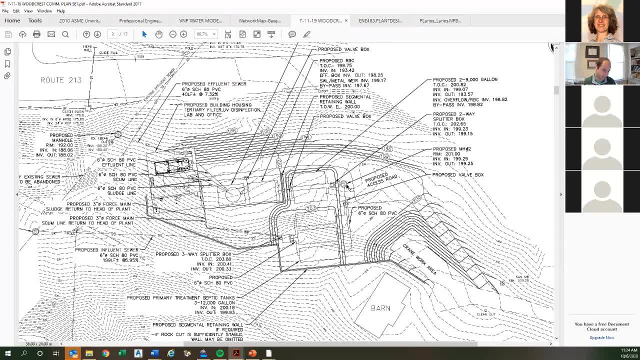 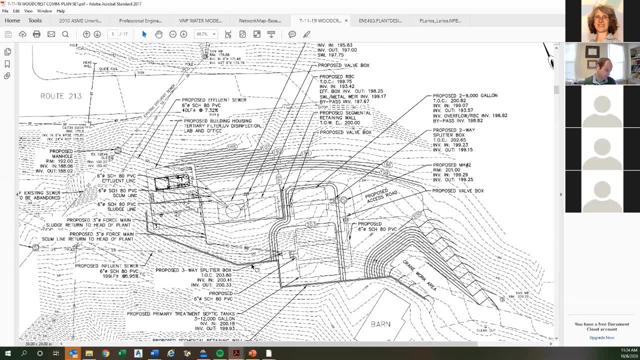 And a big part of this is working with the topography. Where can you place things? Where can you stage construction equipment? How can you get you know? how can you get a sewer at a certain slope to you know? get to this elevation. 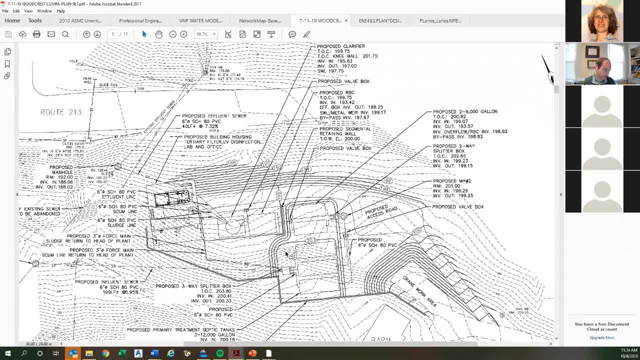 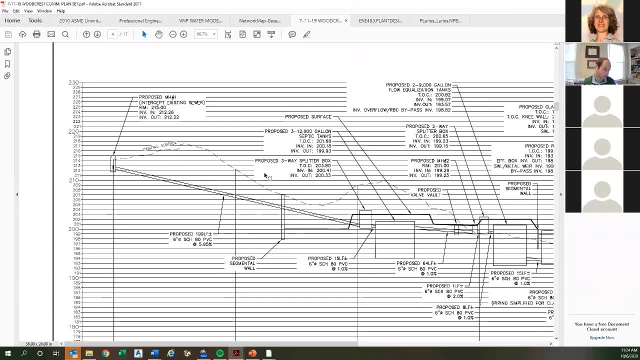 So you need to be creative and move things around and iterate until you've got it. And, as I mentioned before, you're showing hydraulic profiles, So you know if you're going to have a lot of water, you're going to have to have a lot. 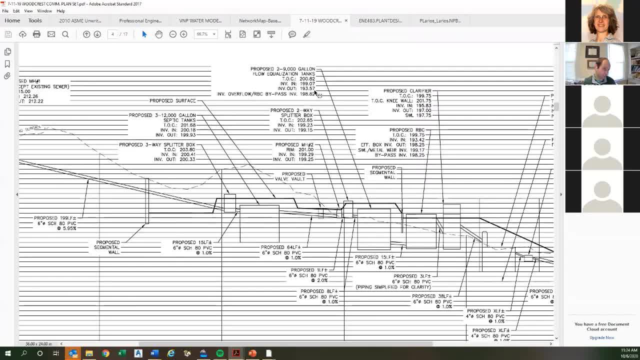 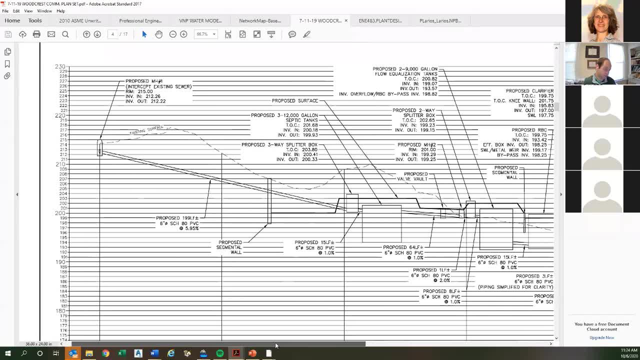 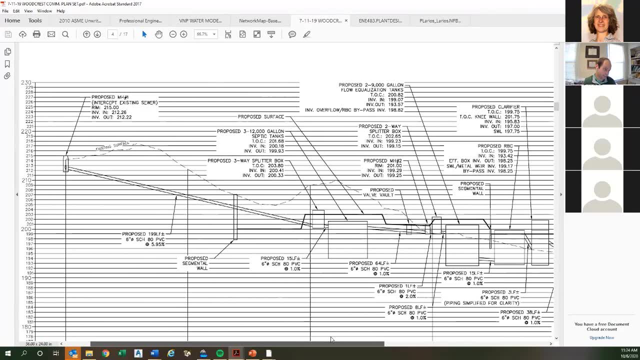 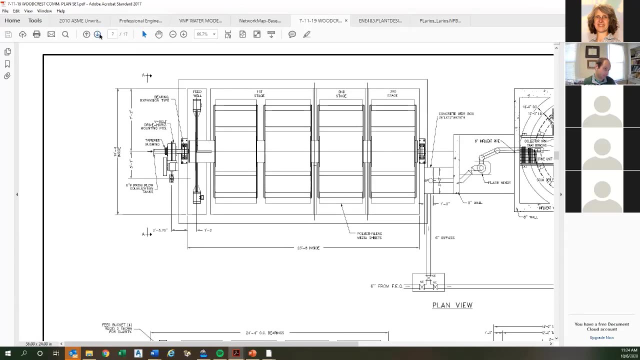 of you know, top of concrete of the tanks, invert elevations and water surface levels throughout the, you know, from the influent sewer to the effluent sewer. So that's all fluid mechanics and hydraulics applied And then you've got schematics, details of the RBC units. filter building flow equalization. 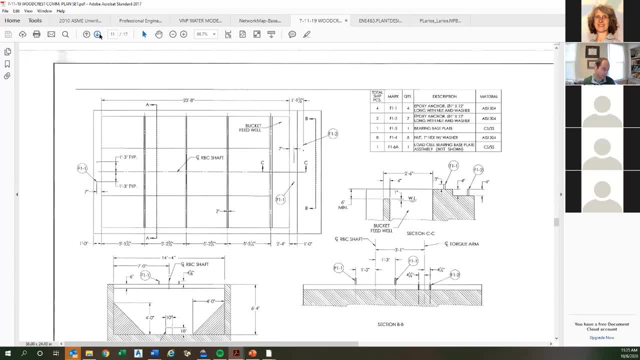 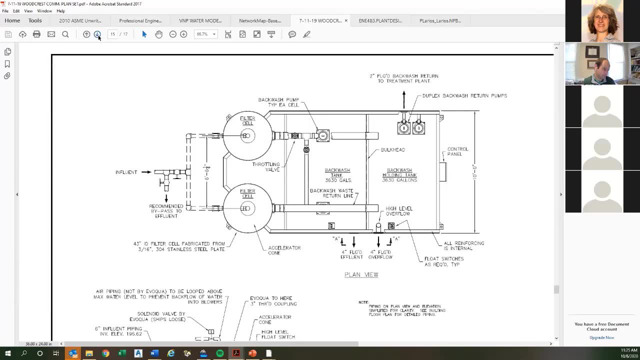 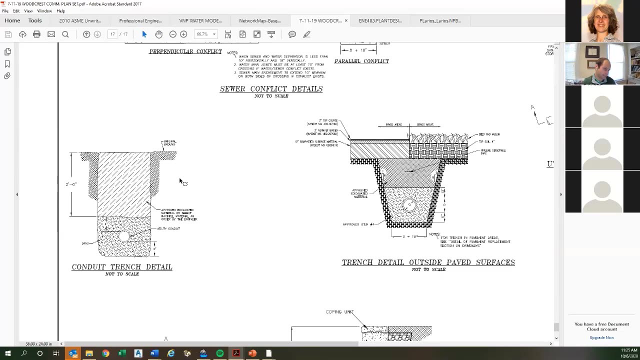 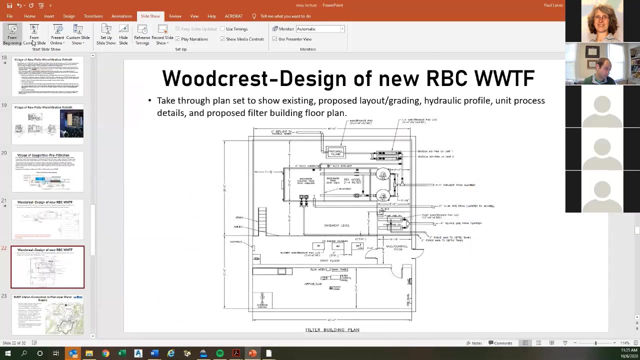 etc. That looks like the RBC clarifier filter UV. So everything that was a preliminary plant set sent to the DEC. They actually, I think, pulled their permit due to COVID or their application. One last one. 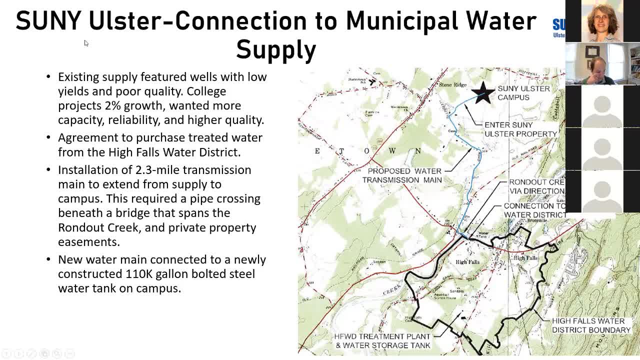 This is primarily treatment. but SUNY Ulster had low yields in their wells and poor quality and they project growth So they wanted to connect to a municipal source. High Falls Water District here on the map actually taps into one of the aqueducts from 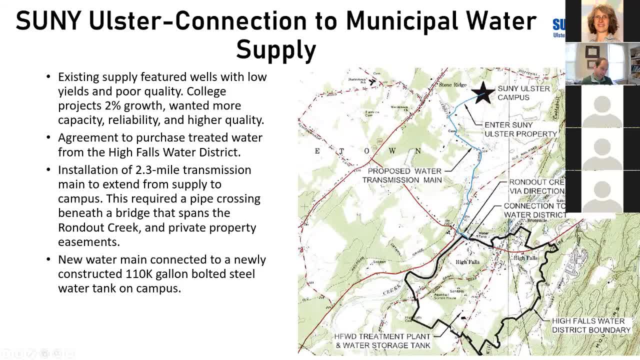 New York City, But they treat it way down here and this is where the water district ends. So that's where The college agreed to buy water from this district and tap in there, And then they had to run a 2.3 mile water transmission line to campus, which required. 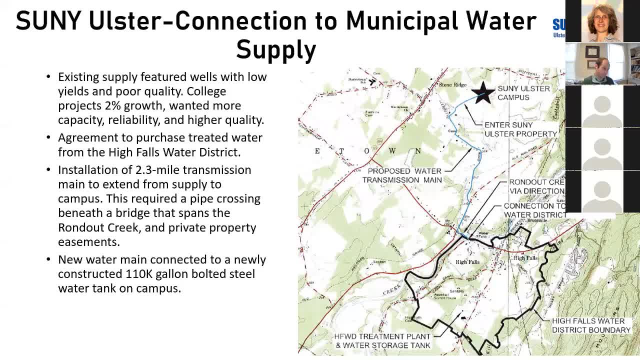 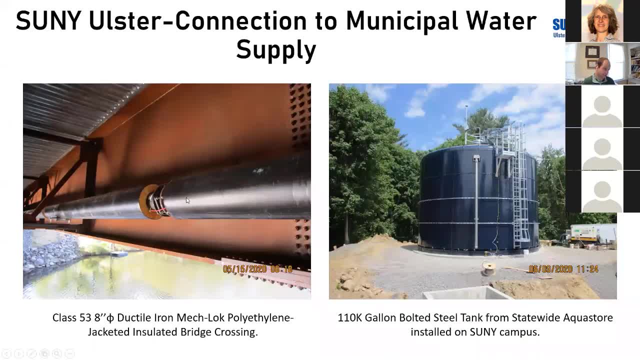 a bridge crossing and some private property easements and then a new storage tank on campus. So here's a picture of the bridge crossing under the Above the Roundout Creek. Okay, And that's a lot more difficult than it looks. 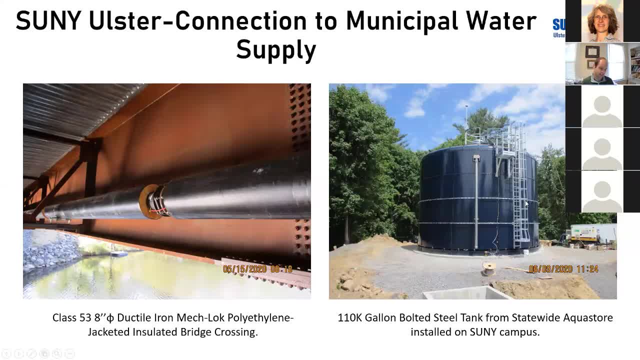 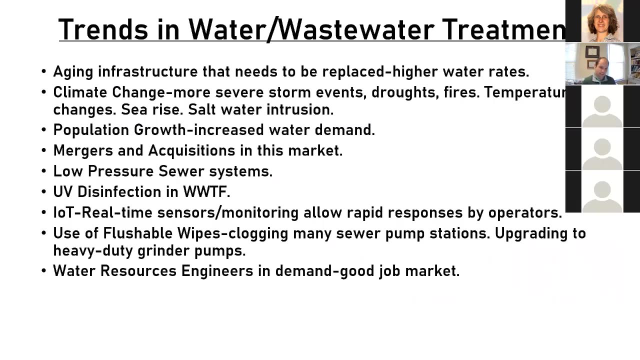 And then this bolted steel tank is so that they can provide gravity distribution to campus with their new water source. So am I going long here? I could skip this Well aging infrastructure, Fleeting hydroelectricity, Okay, And higher water and sewer rates. 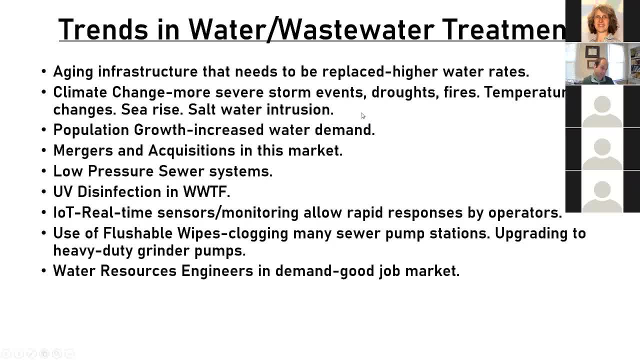 That's been happening for years and it's gonna keep happening. Climate change: We have more severe storm events, droughts, fires- Everything happening in California is showing that. Temperature changes, sea rise and saltwater intrusion: These are all affecting our water. 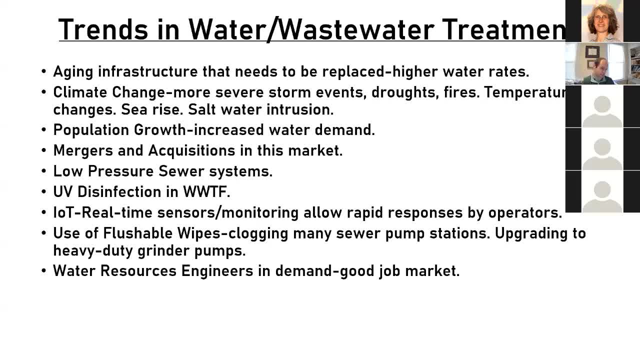 Population growth is increasing demand Mergers and acquisitions. a lot of the big players in this market are buying out smaller firms like us To get more of a market share. Low pressure sewer systems are becoming somewhat common, to lower cost if gravity is not feasible. 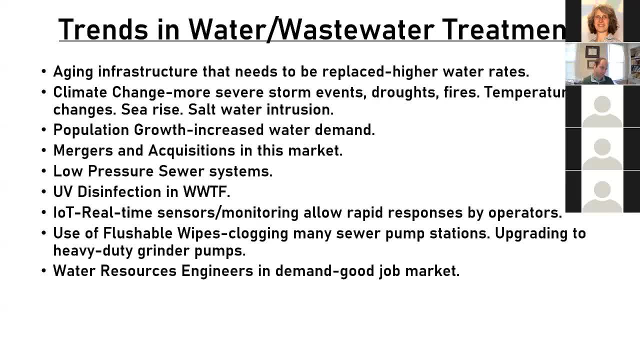 UV disinfection and wastewater treatment. I mean, I don't know if that's a trend. I think it's been going on for some time. I just find that all of our jobs we're doing that. That's because they don't like having a chlorine residual in the receiving water. 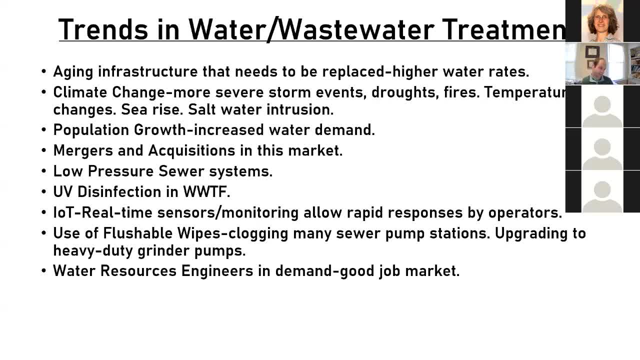 And we're doing that Just to give you an idea of where it's going. But no, we're just trying to get things moving. We're trying to get things moving. That's more than we can. The other thing we're trying to do is stop that transition. 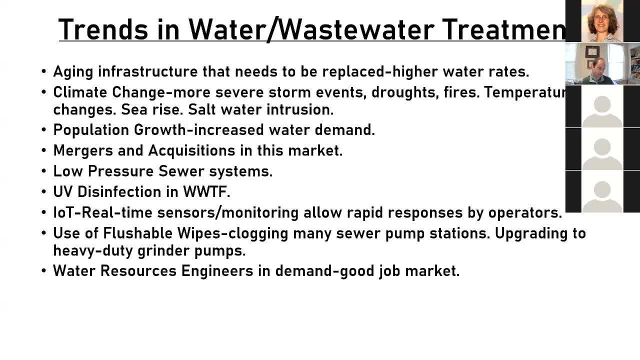 Don't leave it in the water, Just get it up to a minimum level. We need a lot of equipment. We need to get the water to the level If we want to get it up to a standard level. get it out of that mix. 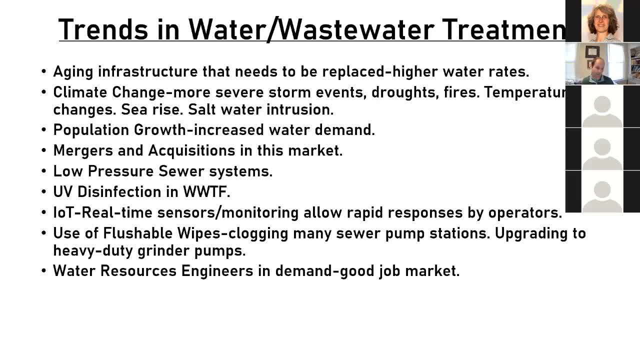 We need to get it to a level where it can generate oil. We need to get the nitrate to aroma. We need to get it over to the sink. Right now we're looking at gas and we have a lot of fuel. We've got a lot of oxygen going. 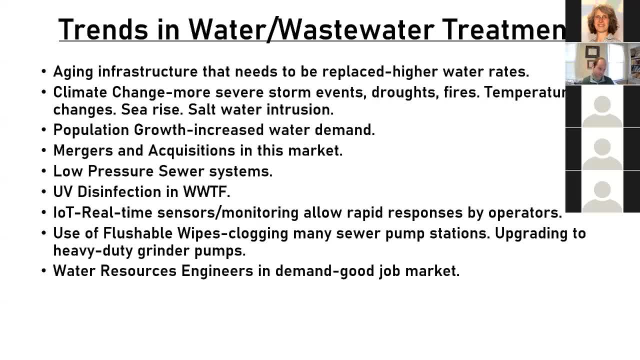 But we're not doing that. We're not doing the oil when something's wrong at the plant or they're not meeting a standard and adjust rapidly. Funny enough, the use of flushable wipes has made a big comeback and it is clogging up. 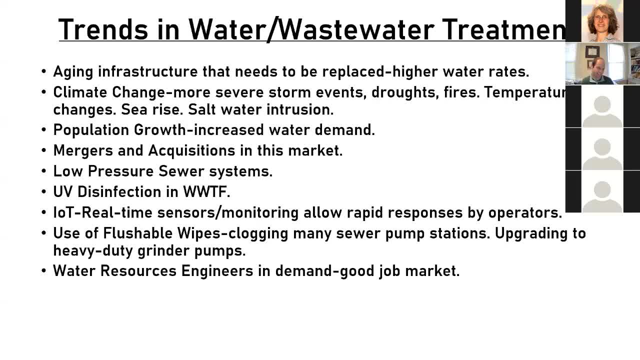 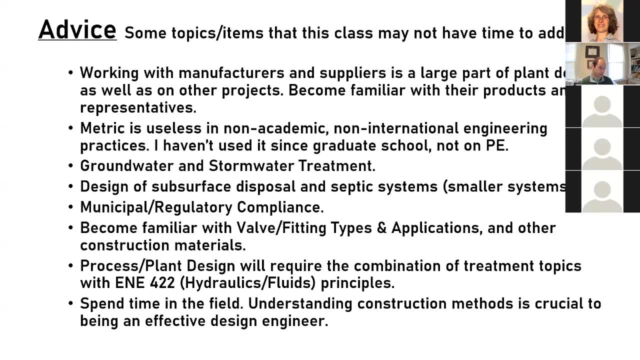 many of our sewer pump stations which we've upgraded to heavy duty grinder pumps. And, yeah, your water resources engineers are. it's a good job market. you're in high demand. So some advice I can offer from my seven years since I've been in your seat. 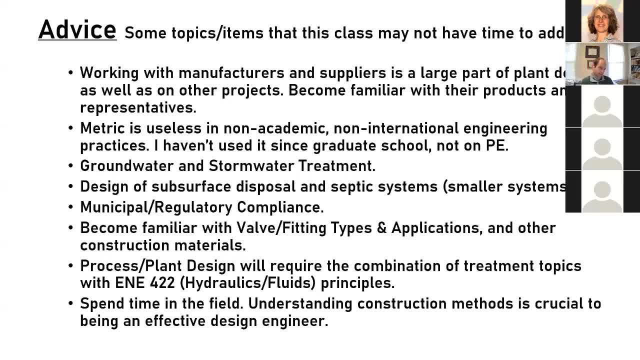 working with manufacturers and suppliers is a large part of plant design. They'll supply drawings of, I mean, anything you get. it needs to be made by a manufacturer. So when we get an RBC unit or a clarifier, we're ordering it from a manufacturer. 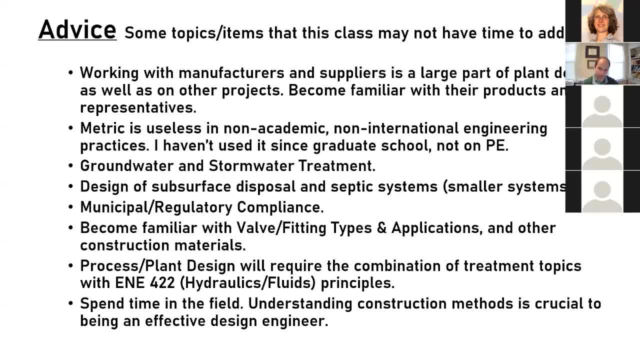 and they're supplying. you know drawings to be edited by us and make work with the hydraulics, But that's a large part of it. Metric, I haven't used it since school. Don't think I will. It wasn't on the PE. 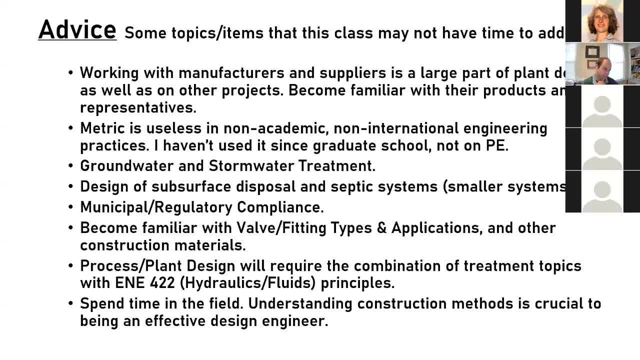 That's the only qualm I have with the textbook that you guys use Design of subsurface and set, you know, residential septics Systems. you guys will be able to take up on that stuff quickly if you know all this. but man, this class doesn't have time to get into that. 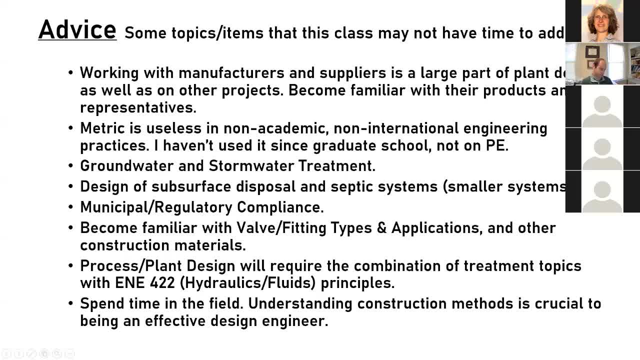 Familiarity with valve and fitting types and applications, other construction materials. that'll help you be a better designer and control flow. Obviously, and like I've said a couple of times, combining it with hydraulics is key And spending time in the field. 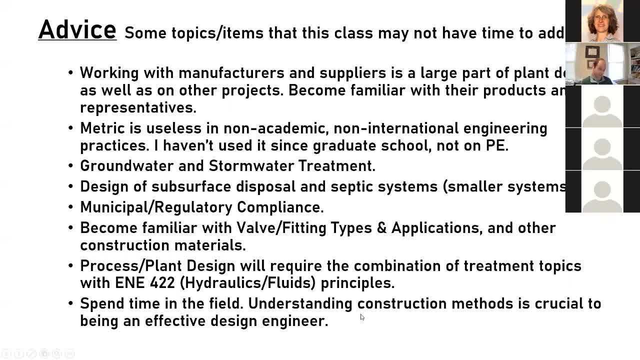 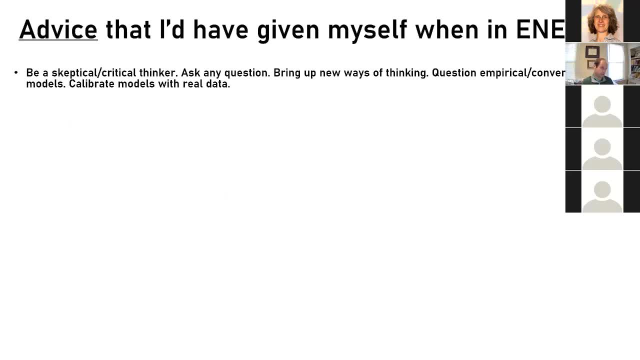 Spending time in the field is key To understand construction methods. if they're gonna build it differently anyways, then there's no point in designing it. So spend time in the field. Advice that I have given myself in 483, be a skeptical, critical thinker. 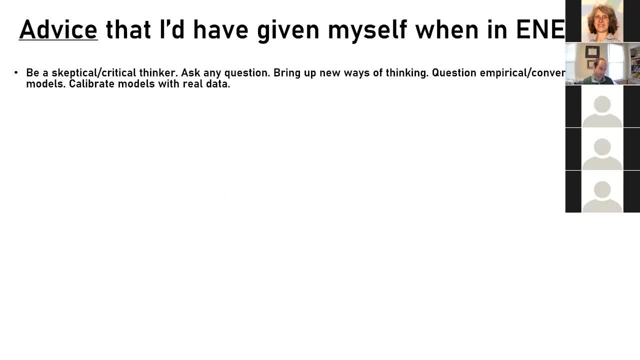 Don't be scared to ask any question, or else you're not gonna learn. Don't be scared to bring up new ways of thinking. Question empirical and conventional models. Don't be scared to ask any question, or else you're not gonna learn. Don't be scared to bring up new ways of thinking. Question empirical and conventional models. 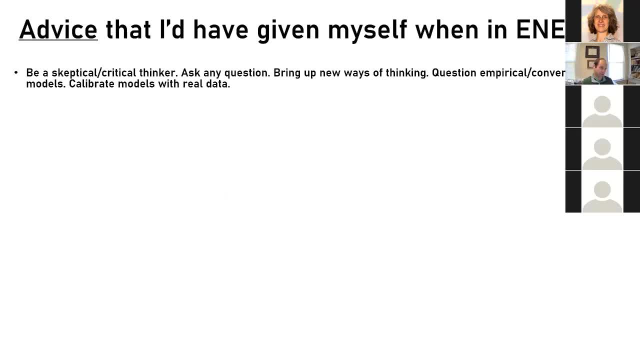 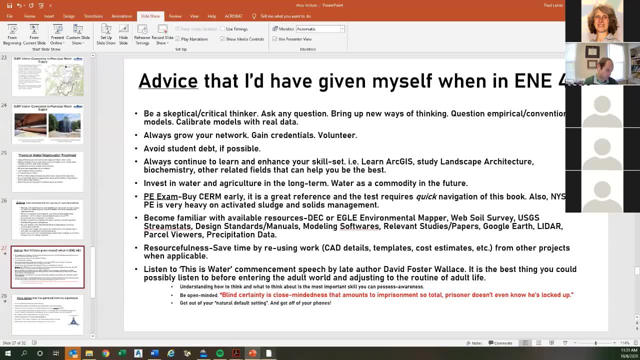 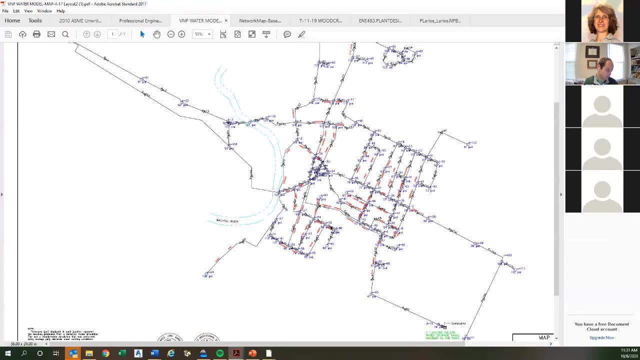 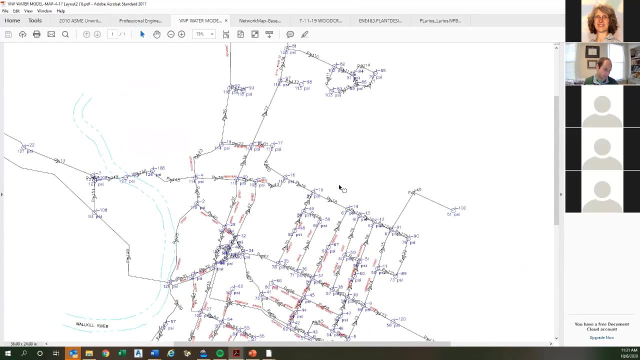 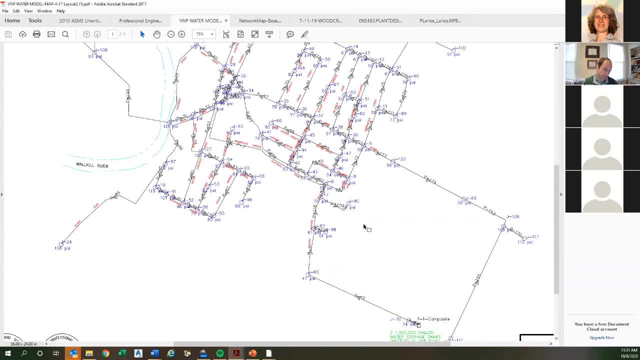 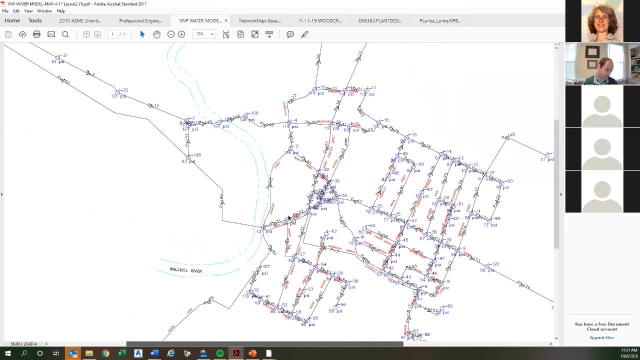 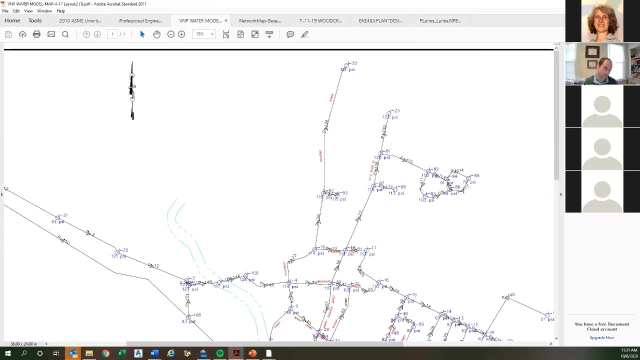 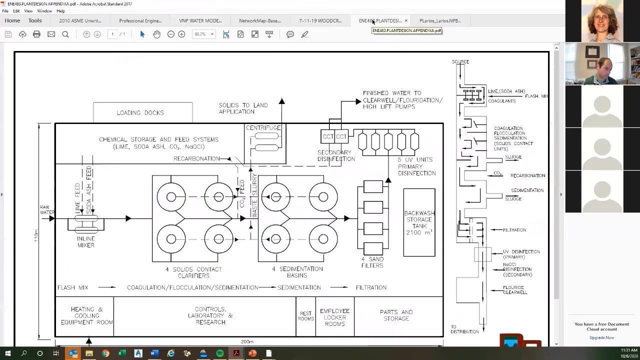 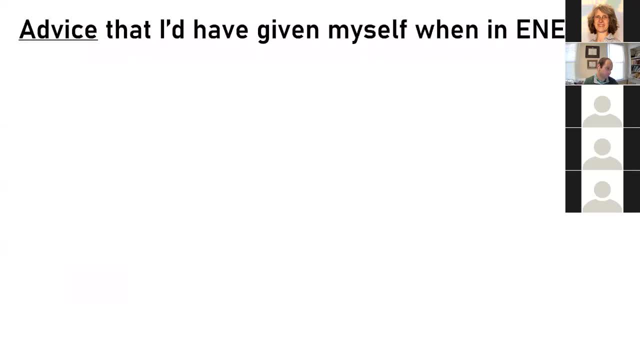 Always grow your network, gain credentials and volunteer in your community if you have time. Networking is huge. Gaining credentials, joining professional organizations such as ASCE- I'm in the NSPE Society of Professional Engineers. You could try to get published or get on a board of one of those. 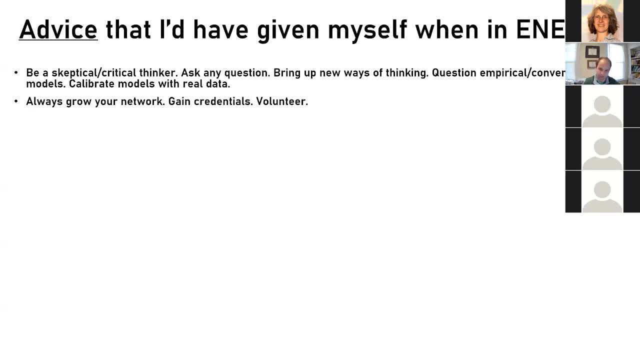 I volunteer at our local YMCA on the board of directors. It just it's important to be involved in your community and it helps business too. People see that and they want to help you too. Avoid debt if possible. High interest debt can be crippling. 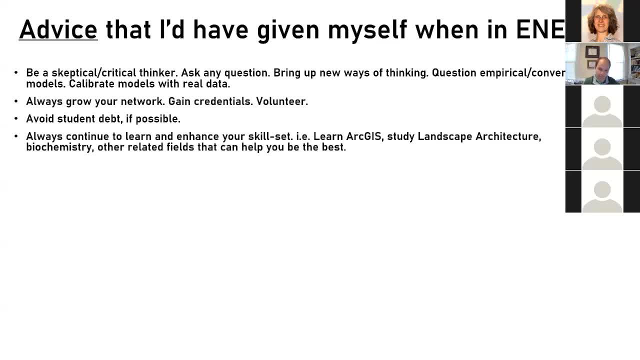 Always continue, Continue to learn. You will have continuing education requirements once you get your PE, if that's your plan, But I you know. outside of that, I've been trying to learn ArcGIS, which is a very powerful tool nowadays. 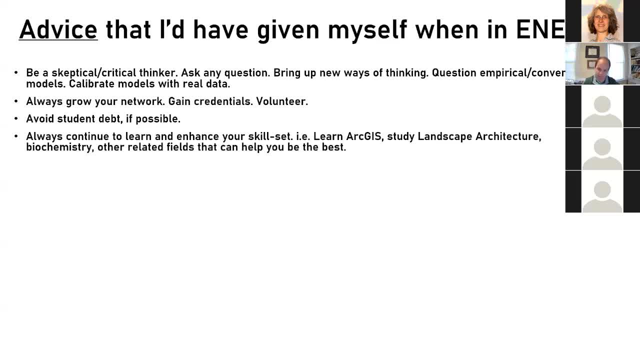 They didn't teach that back when I was in school. I've been studying some landscape architecture, any related fields that can help you be the best. It's more of a personal thing. I like to invest in water and agriculture. I'm not a big fan of agriculture. I'm not a big fan of agriculture. I think water prices are just in the future are going to be a lot higher, And there's a lot of water groups that are publicly traded now, or even infrastructure, like Xylem, People that make pumps and you know manufacturers in that sector. 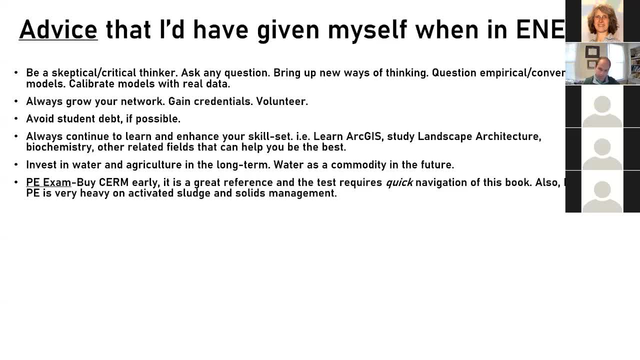 PE exam, So this one I'll spend some time on. I've always I pride myself on how good of a test taker I was. I took the FE. They give you two four hours for both halves, just like the PE does. 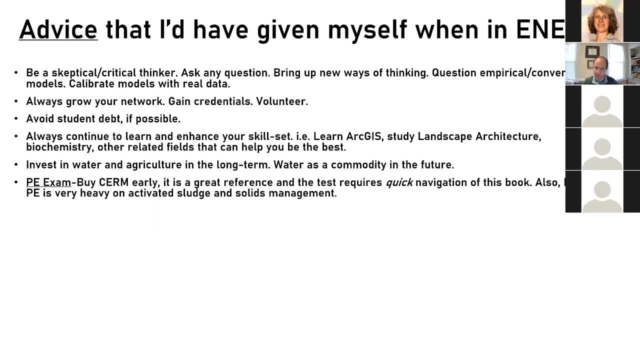 I didn't study for the FE because Dr Mastin's capstone design project was due the day before. But I was so used to solving problem sets every day back then that I cruised through both halves in two hours Out of the blue. 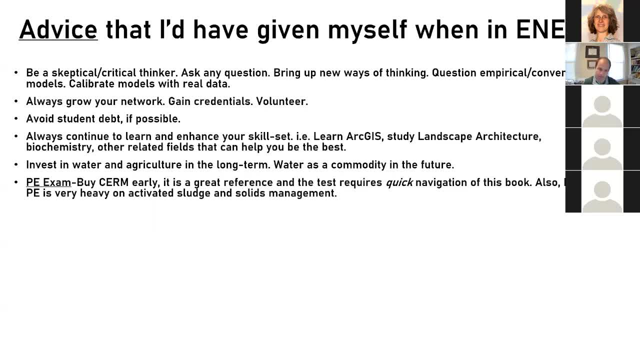 Out of the four And never had a doubt. PE exam I might have been a little cocky. I did fail it once. I did not have the correct book because I started studying so late that I didn't even realize. It was really embarrassing for me. 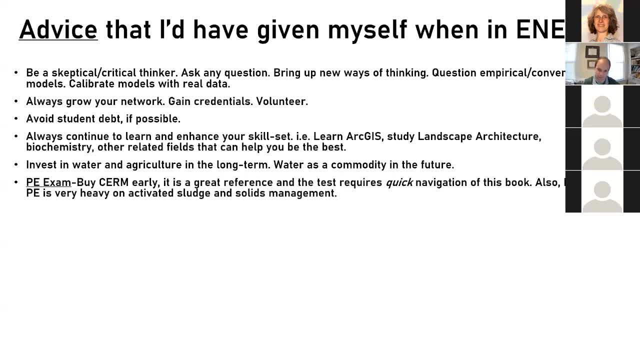 But that's where we learn from our failures. I would you know, I would suggest buying the civil engineering reference man, Which is right here. it's 90% of the test is out of this book. I took it the first time without it. 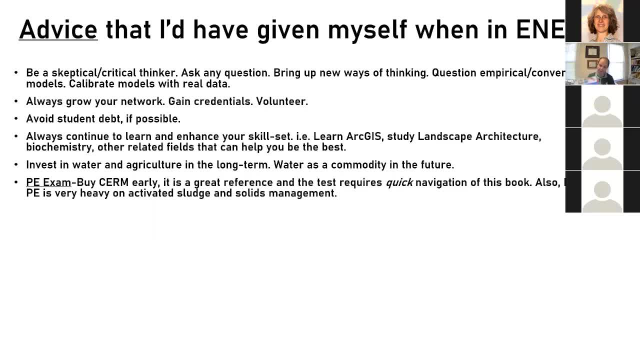 I had. I was flipping through all kinds of books and running out of time. I mean you can buy it right when you start practicing, because it's a useful reference And then you'll be able to navigate the book. So I've been letting our our new, junior engineer use it. 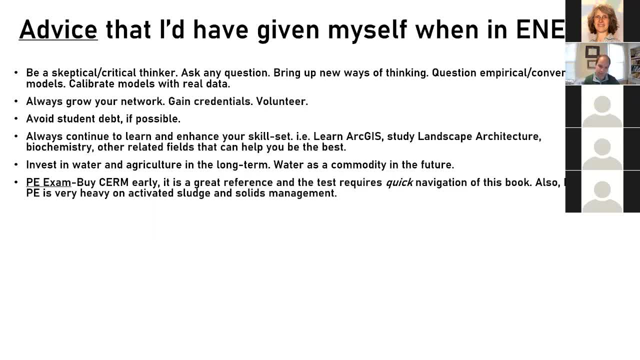 And he by the time he's done it, he's done it By the time he takes a test. I think he'll be familiar with it and not even have to study as much. And also in New York, the PE both times was very heavy on activated sludge and solids. 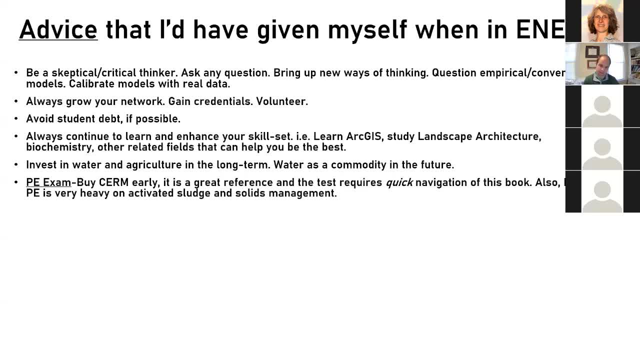 management, for whatever reason, They really like to drill you on that stuff, You know. become familiar with your available resources: environmental mappers, web soil survey, stream stats, all the design standards and manuals. Yeah, So there's a bunch of great resources. 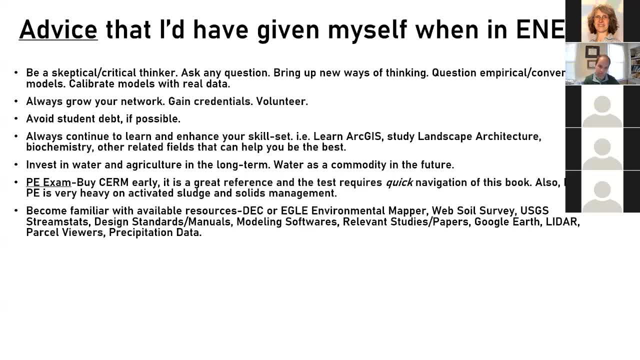 There's a bunch of great resources. There's a bunch of great resources: Google Earth, LIDAR, parcel viewers and precipitation data, to name some. There's many more. There's so much available on the web nowadays: Resourcefulness, save time by reusing work and such as CAD details, templates, cost submits. 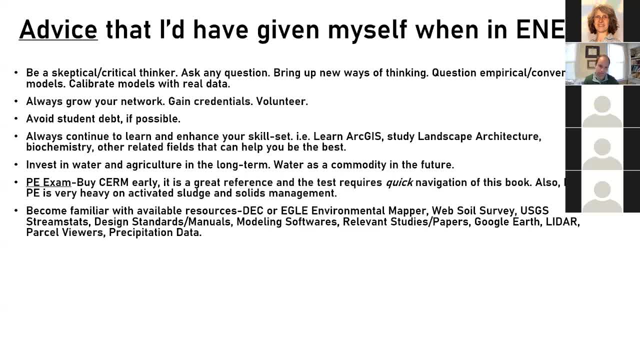 from other other projects. This is huge for us and saving time and being able to bill less to the clients. It's more of a personal thing. Listen to. this is water. It's a commercial water, but it's a commercial water. I'm just going to use it as a personal thing. 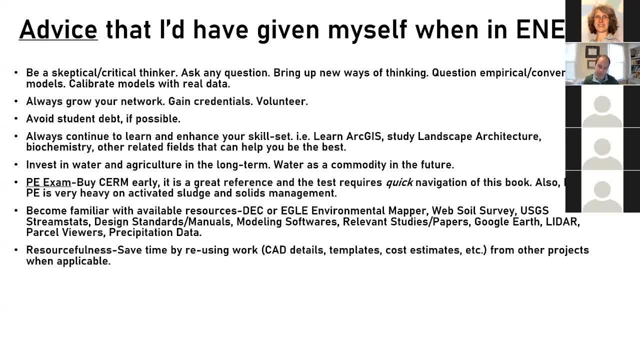 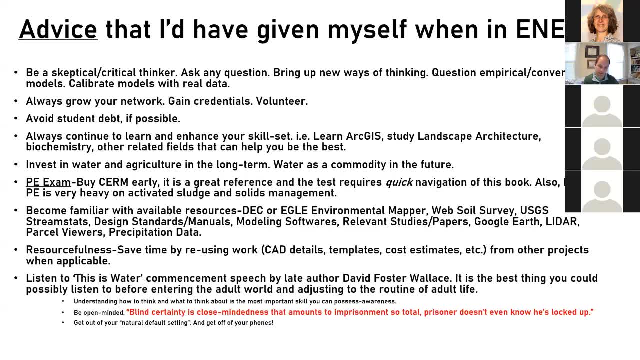 And then you can use it as a research material. But it's also a kind of a you know a product, Smith from other other projects. this is huge for us and saving time and being able to bill less to the clients. it's more of a personal thing. listen to this. 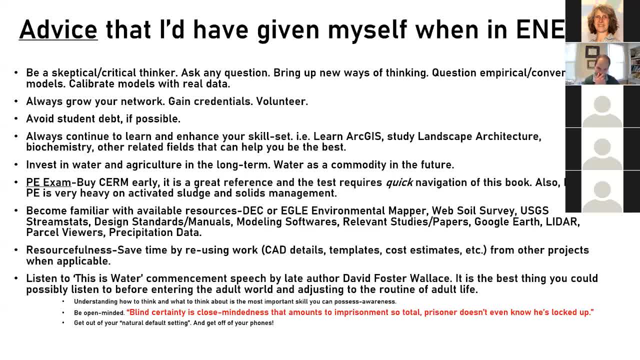 is water. it's commencement speech by the late author David Foster Wallace. I highly recommend that you all listen to it. it's the best thing you could possibly hear at this time in your life. I have a link to that on the last slide. um, I highly encourage that. more advice, just a few more track and build time. 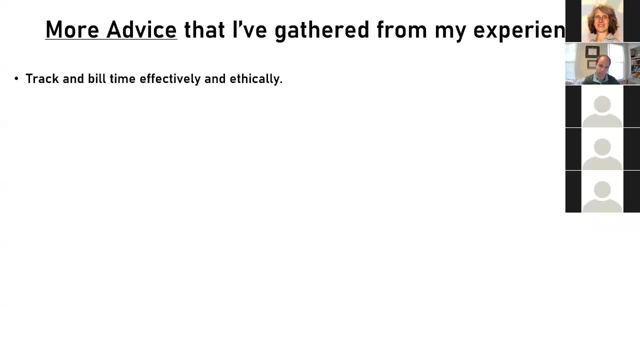 effectively and ethically. I know dr Messon likes to hit on the ASCE ethical canons. I'm sure one of them has to do with- you know, not misreadings- representing your time. I'm not sure, though. keep records on all projects and coursework, if you don't already. I started doing this as a freshman and it 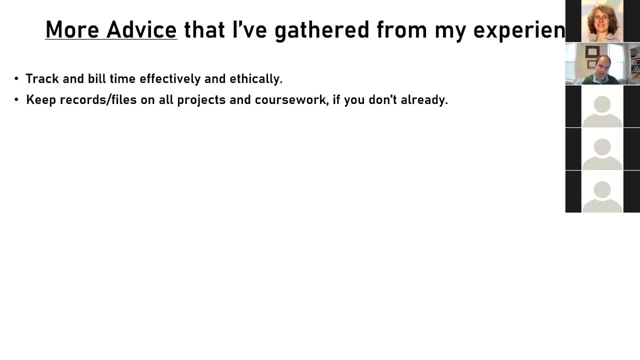 enabled me to you know trade. you know I had a bio test. do you? did you have this professor? I'll trade you this, this old bio test, for you know this homework and then keep you know it. it's kind of resourcefulness, but also for your PE app. 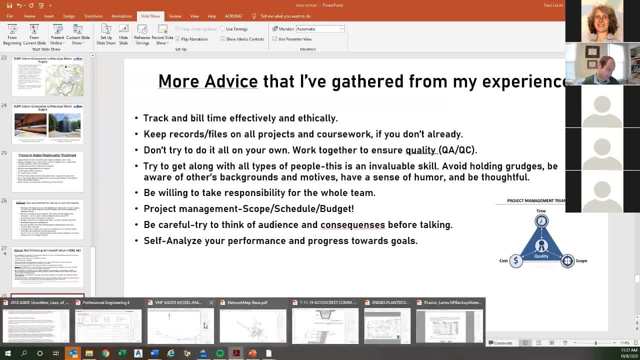 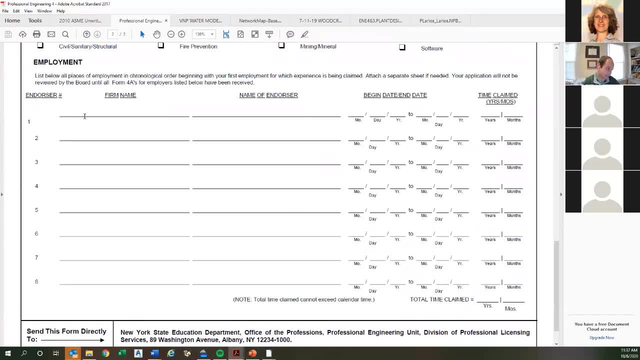 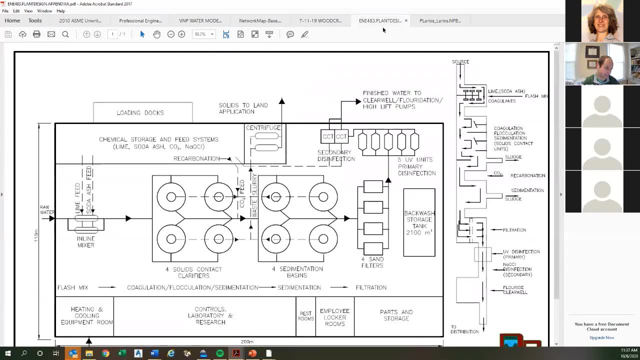 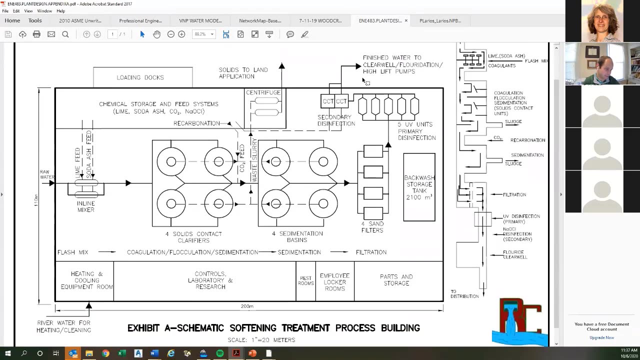 you'll need it because you have to list, as shown here, how many hours or years and months on every project you've worked on and, as far as saving work, I obviously do that. here is my final project for 483, which was incorporating MSU into Lansing's. 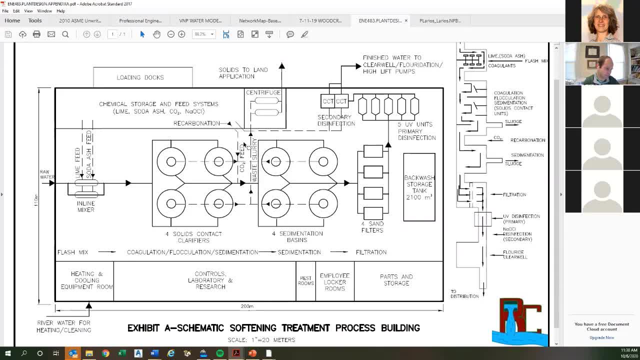 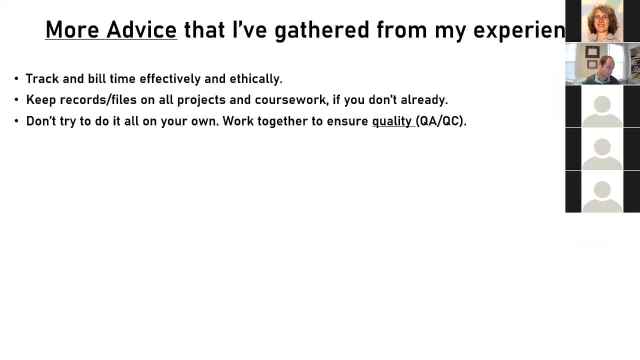 treatment plans? a good question. you can addل and plant, I believe softening plant. don't try to do it on your own like I did on that project I this happens to me too much. it's important to work together and ensure quality. you want your product. 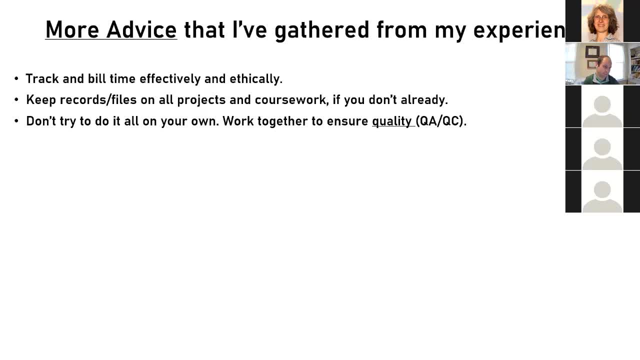 to be quality. so work with your staff for QH. you see, quality assurance and control and other ideas can always help. try to get along with all types of people. this is an invaluable skill. I find that my dad, who's my boss, is great at this. avoid holding grudges. be aware and conscious of others. 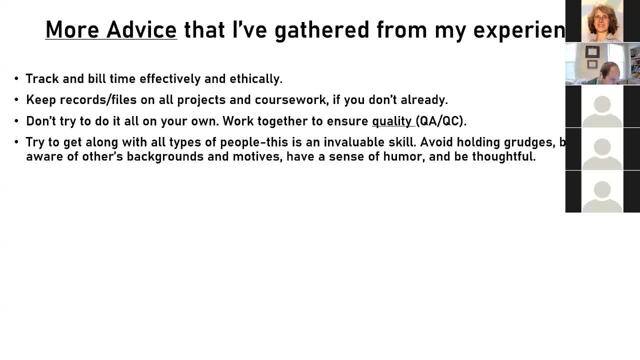 backgrounds, motives and have a sense of humor. try to be thoughtful. this will help you, not just in profession but in your life. be willing to take the responsibility for the whole team and you: project management, scope, schedule and budget. uh, if you take construction engineering, you'll learn. 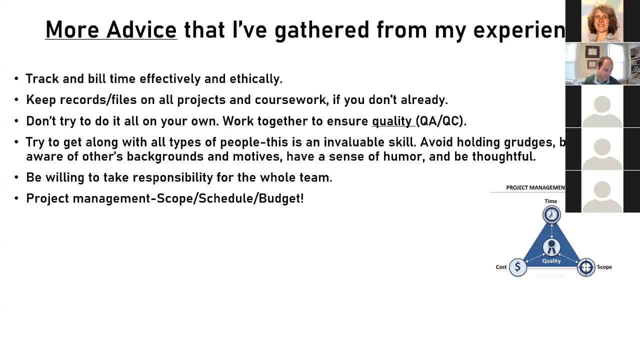 that, but uh, the fourth thing is managing the contractor, because a lot of times the contractors will try to cut corners or make field changes. so you really need to make sure that they are doing it right and as designed. but sometimes they're right and you you can approve field. 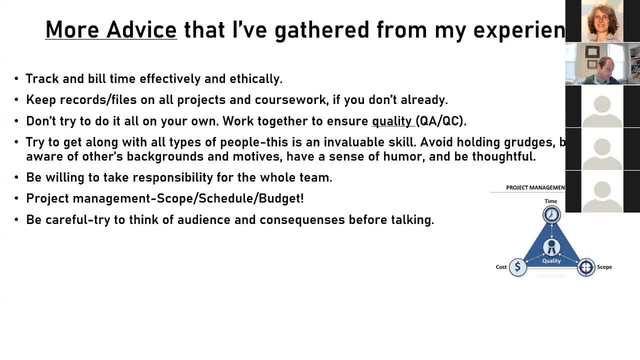 change. um, be careful, try to think of your audience and and the consequences before talking. this is something I've been trying to work on. and another thing that reminds me of my dad: um, I always thought that he was just a slow storyteller, or maybe. um, it took him a while to talk, but now I realize I'm. 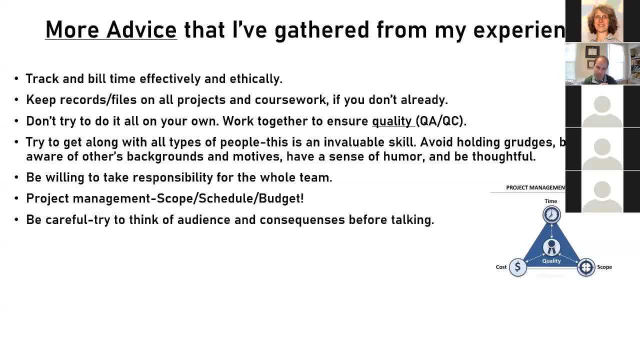 you know I'm watching him talk in front of a planning board and a public- you know- audience that he's really just considered considering the best way to present the information. so if you have to talk slowly, try to do that. um, self-analyze your performance and progress towards goals. I think it's important to set goals. 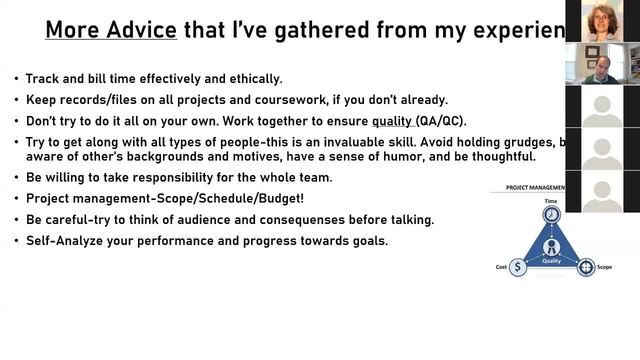 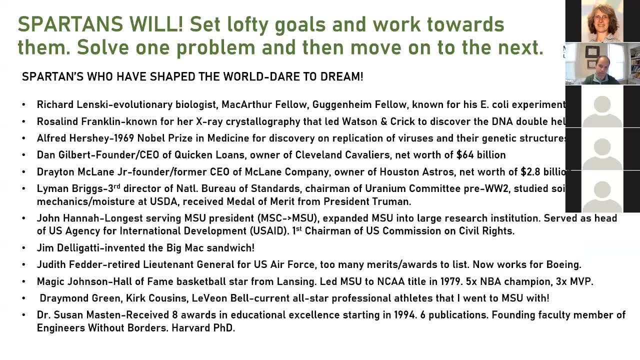 and to be self-aware. um, and that's about it, Spartans will. so here's some famous Spartan alum that can inspire you. uh, dare to dream this. uh, um, Rosalind Franklin helped discover the double Helix. we've got two professional sports owners, Dan Gilbert and Drayton McLean Jr. Lyman Briggs, um third director of National Bureau of Standards. he. 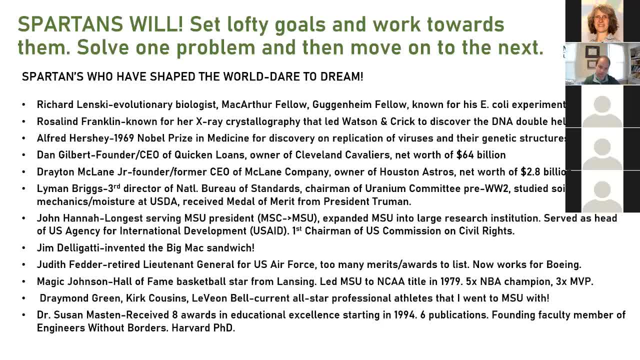 was on the uranium committee pre-world War II, studied soil mechanics and moisture at the USDA and received the Medal of Merit from Truman John Hannah, who I'm sure you guys recognize the name and there's a statue of him on campus. um he really expanded MSU into a large research institution. um headed the US uh in a international 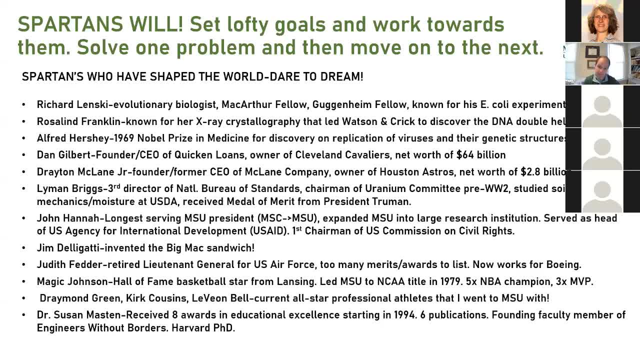 development and was the first chairman of the US Commission on Civil Rights. we've got Jim Delicati, the inventor of the Big Mac. um, I was lucky enough to go to school with Draymond Green, Kirk Cousins and Le'Veon Bell, who were all all-star professional athletes. 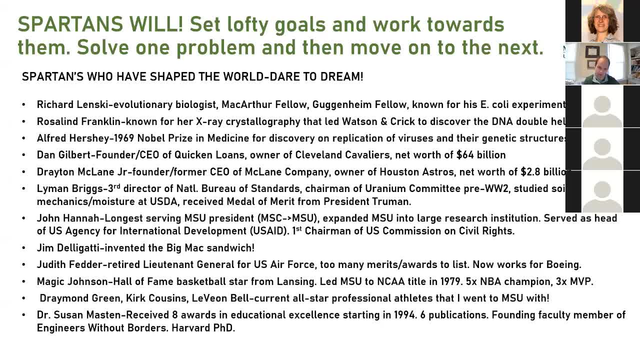 uh, that were there three out of my four years, so that was fun. and then we have our esteemed professor, Dr Mastin. I hope I didn't short you any awards, um, and publications. uh, I got a few more publications. you're good, um, you're with some good company on that slide, um. so yeah, future engineers. 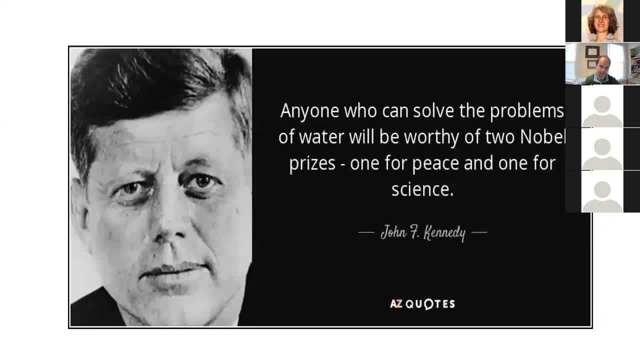 and you can end up on on this slide. one day- and here's a powerful quote from JFK- anyone who can solve the problems of water will be worthy of two Nobel prizes, one for peace and one for science. uh, I'm sure he said that in the 60s, but I'm sure it's still applicable today, as we really still 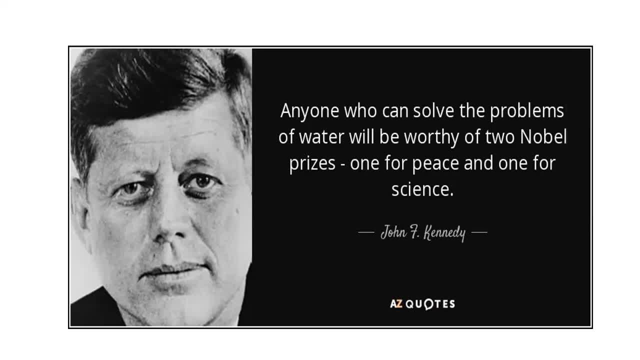 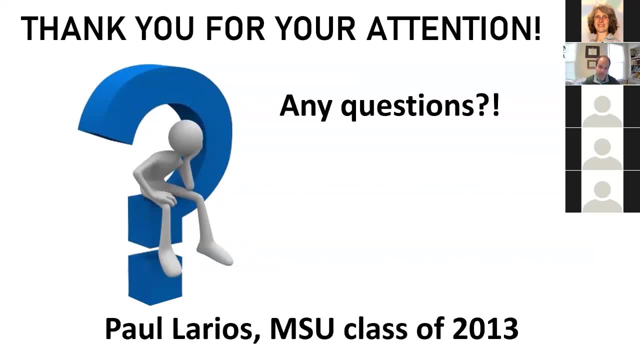 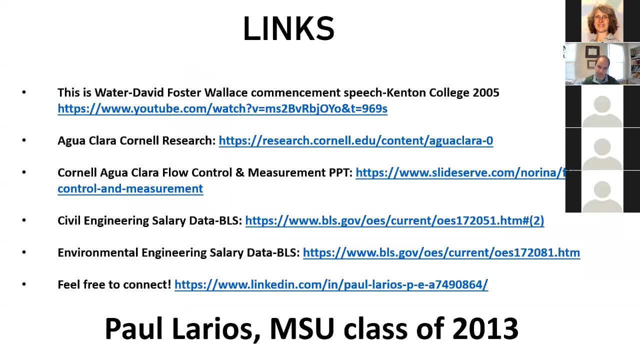 haven't solved problems of water. um, I just thought that was a great quote. uh, any questions class of these folks? If you have any questions, you can feel free to email me or connect on LinkedIn. Dr Mastin can share this presentation with you. I have some links.